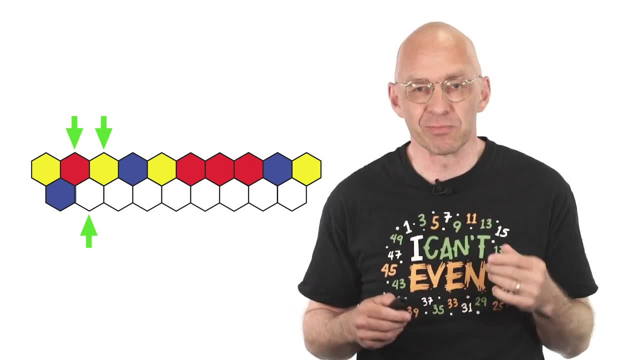 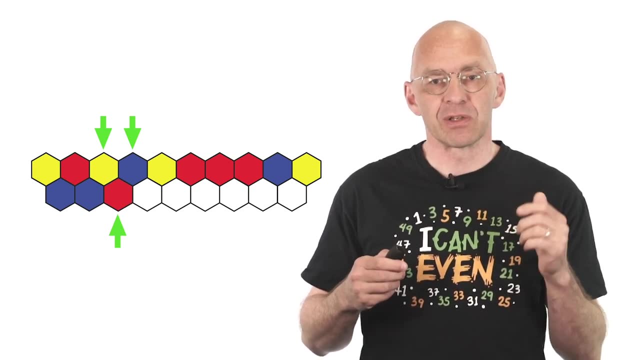 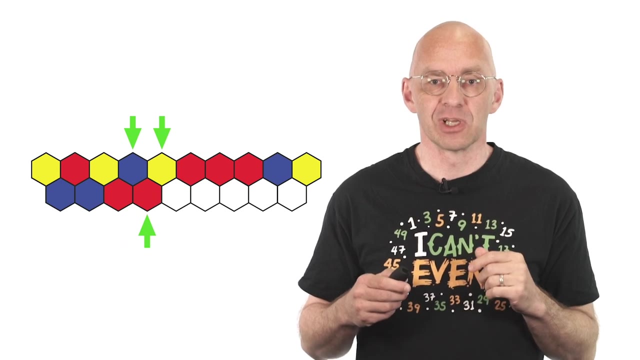 red and yellow, add to also blue. yellow and blue, add to red. easy, right? I'm sure you've guessed already that whenever we are adding two different colors, the result is the third color, and so on: Blue plus yellow is red, yellow plus red is blue. Okay, 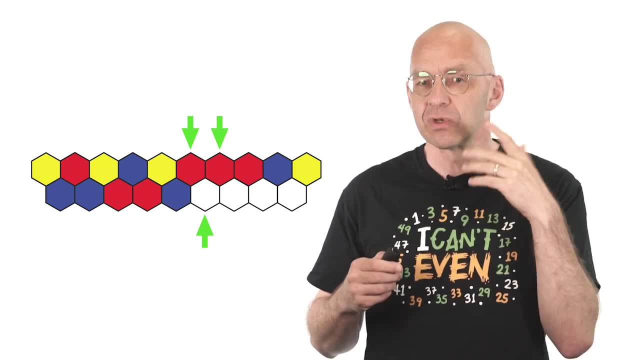 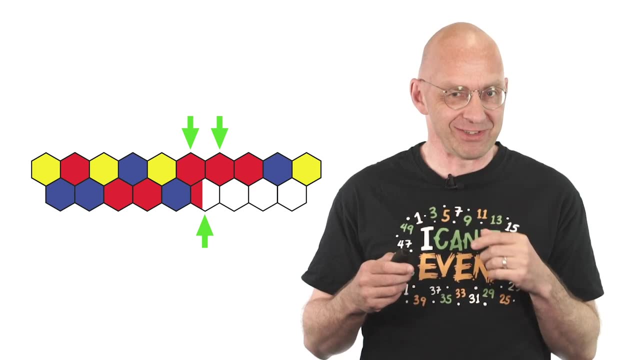 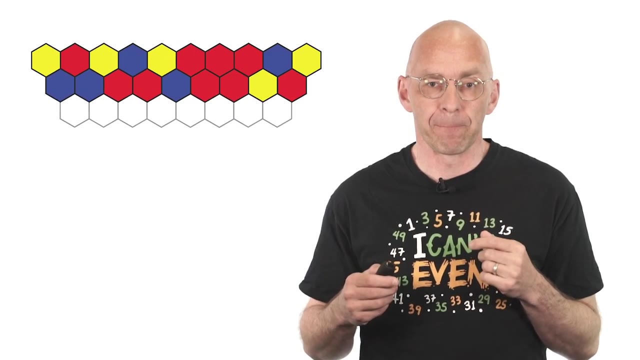 what if we have to add a color to itself? Well, red plus red is red. That's the most natural rule, Agreed, Agreed. Draw a row of eight hexagons underneath what we've got so far And, using the same rules, just keep filling in colors and 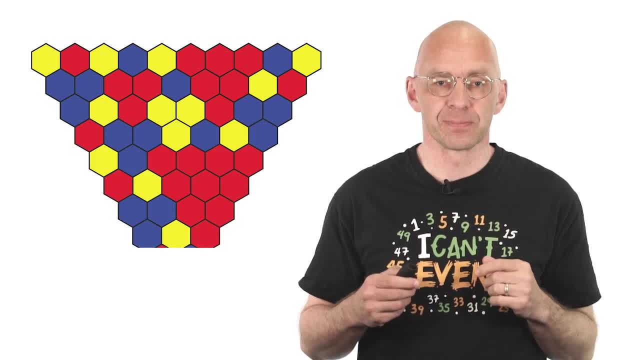 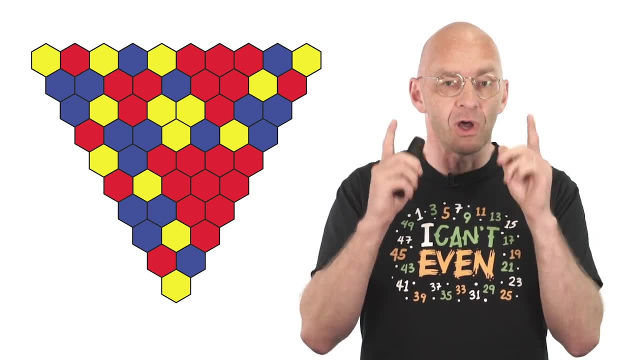 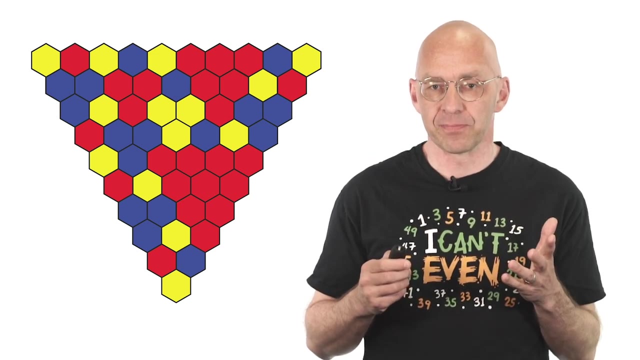 drawing rows until it all ends like this. So you end up with an equilateral triangle composed of hexagons- Important observation: once the colors of the top row have been chosen, all the other colors are pinned down. Here are a couple of examples of triangles resulting from different 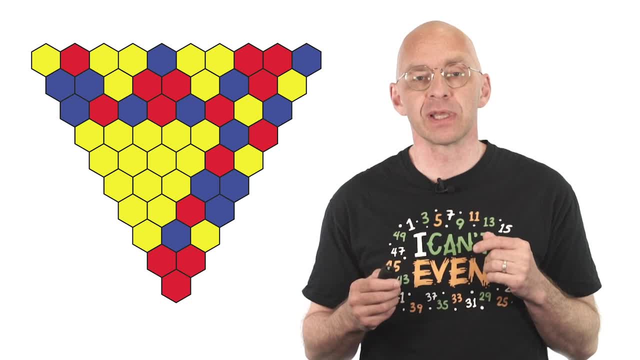 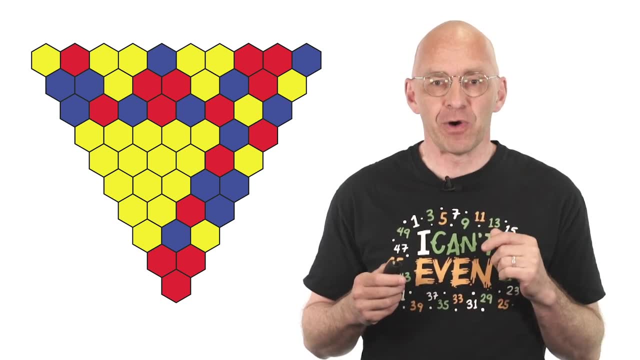 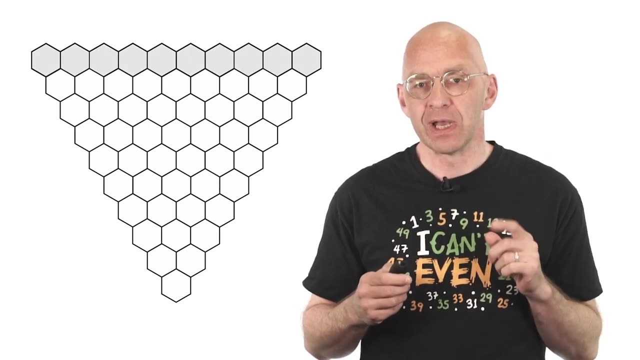 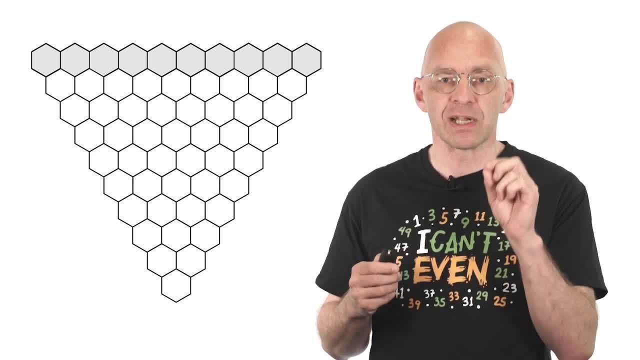 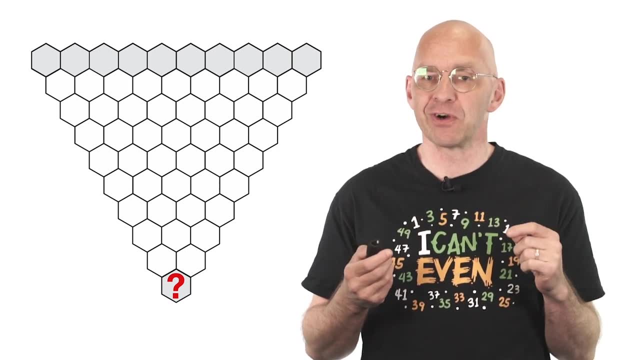 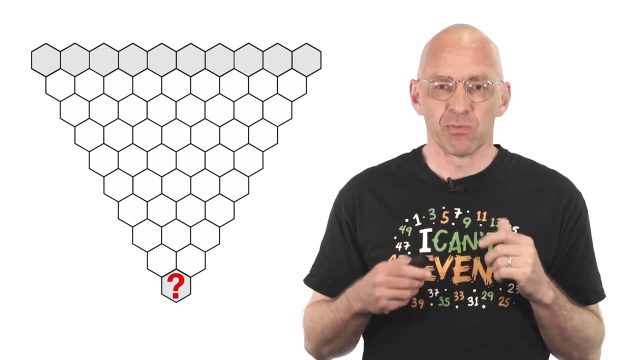 count down from five and ask you to decide what the resulting color of the bottom hexagon is. Get it right and you win a lifetime subscription of Mathologer Videos. Yes, okay, it's free anyway, but you win bragging rights. What are you going to do? Of course, you can just guess for a 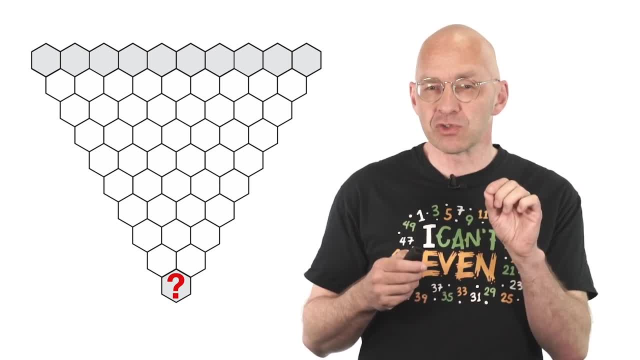 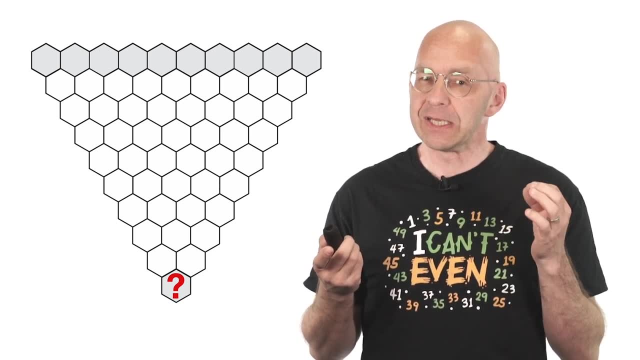 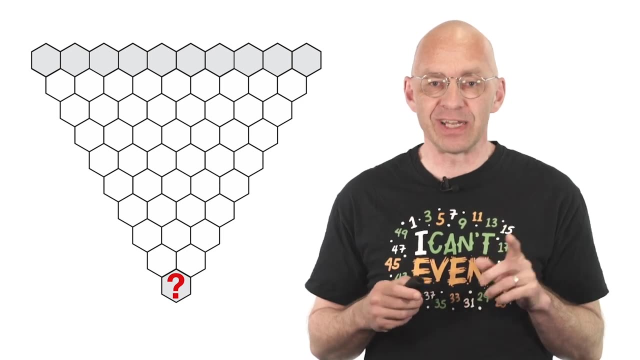 one in three chance. On the other hand, since the first row will determine all the colors of the hexagons below, you can just calculate the color of the bottom hexagon If you're really really quick or if you pause the video. Anyway, time to go Ready. Well, ready or not, here we go, Okay. 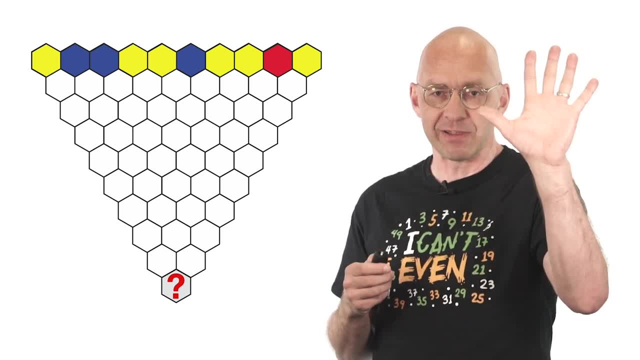 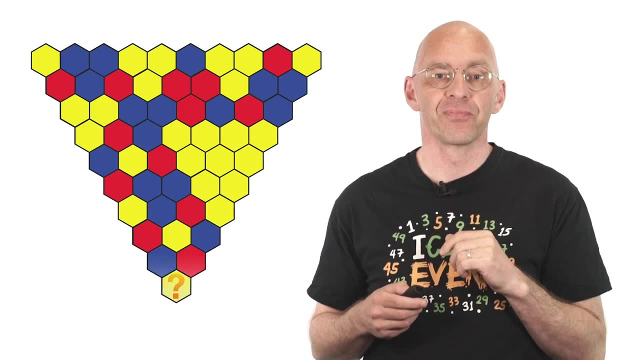 make your guess. What's the color of the bottom hexagon? Here we go. Okay, make your guess. What's the color of the bottom hexagon? Five, four, three, two, one, and the answer is yellow. Did you get it? 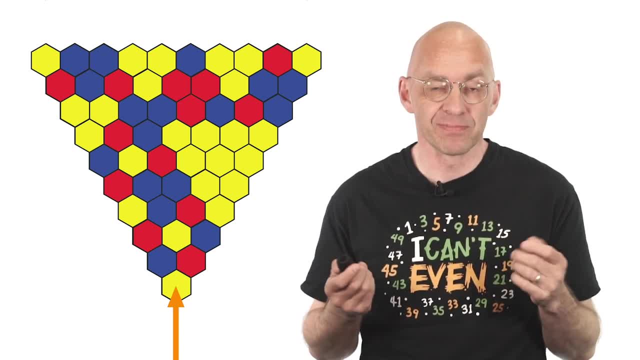 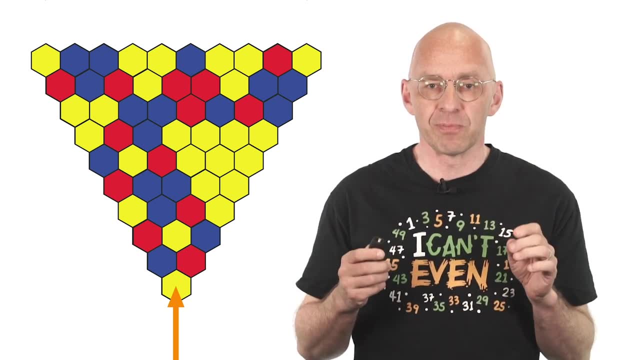 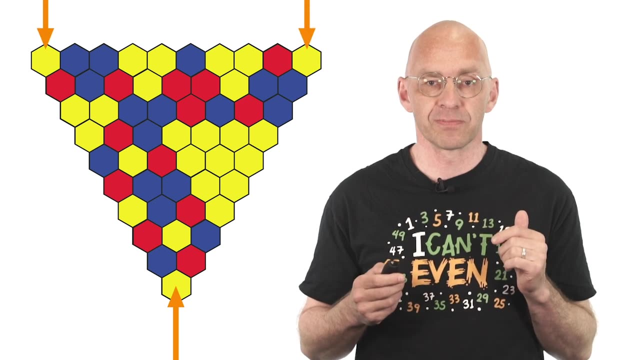 without pausing the video or just guessing, Sounds impossible. Well, it turns out that there is a super surprising shortcut for this calculation. It turns out that the color of the bottom corner of our triangle is simply the sum of the two colors in the top corners. 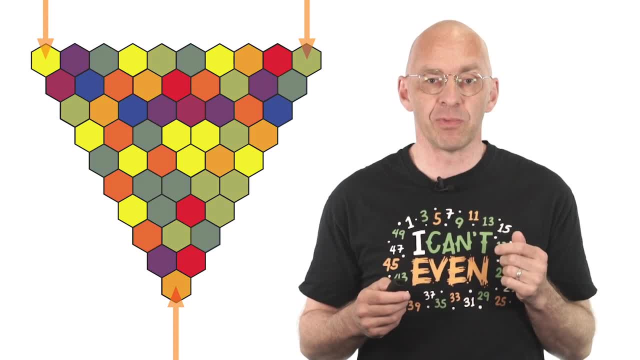 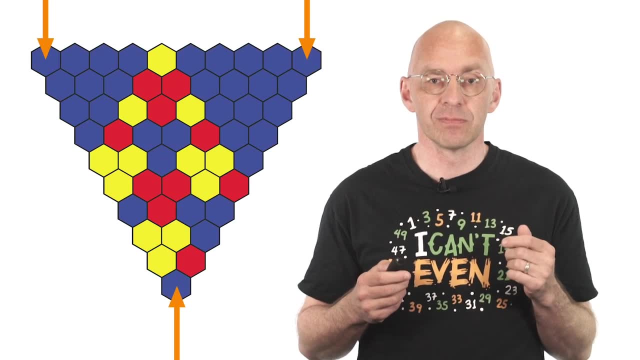 There, yellow plus yellow at the top is yellow at the bottom. Yellow plus blue at the top is equal to red at the bottom. Blue plus red is yellow. Blue plus blue gives blue. It really works Pretty amazing, isn't it? Choosing different colors in the top row gives very different colors of our. 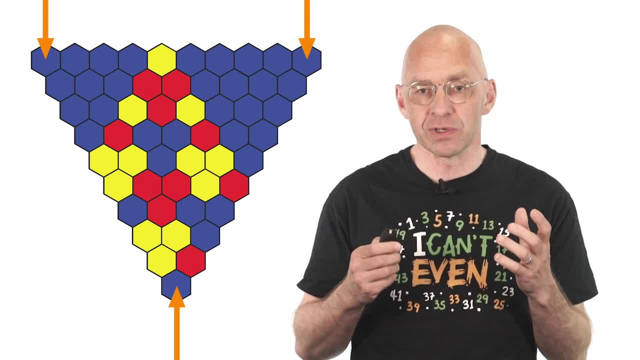 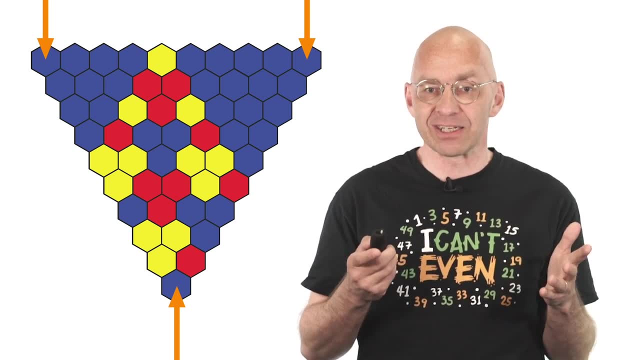 triangle, and yet the colors of the top two corners alone determine the color of the bottom corner. Weird huh. Well, it gets weirder. What if, instead of ten hexagons at the top, we started with nine hexagons? Well then, the 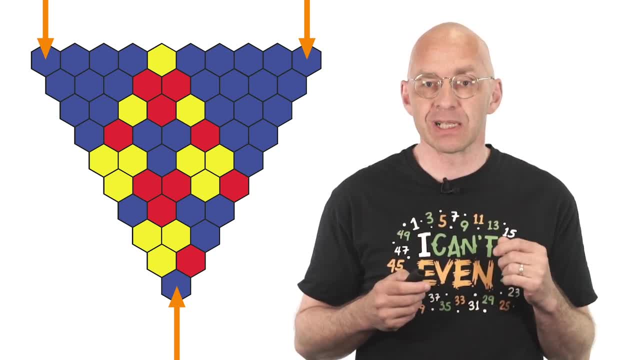 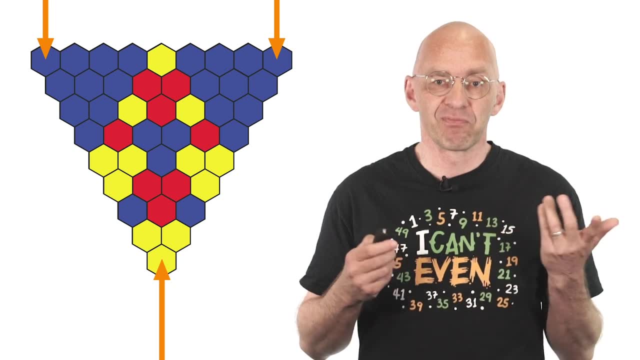 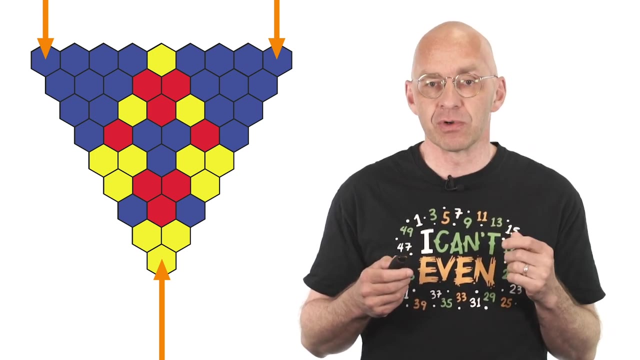 shortcut doesn't work anymore. For example, stripping a slanty column off of the width 10 triangle over there gives us a width 9 triangle, And here the shortcut clearly doesn't work. Blue plus blue should be blue, not yellow. Stripping off another row gives a width 8 triangle Again. 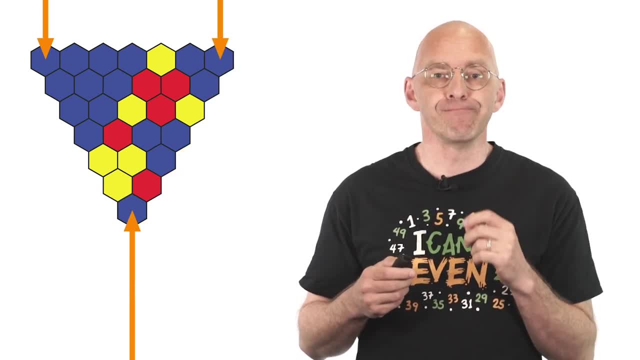 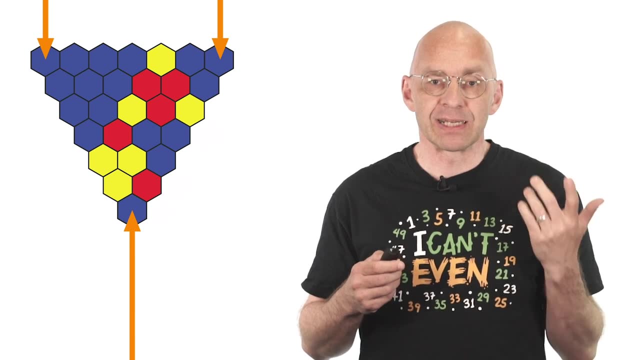 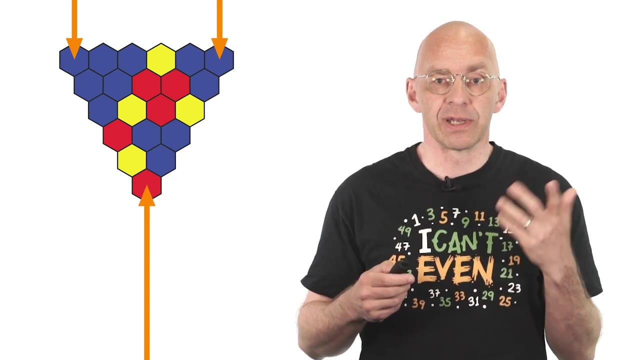 the shortcut doesn't work. Keep on going. Blue plus blue is blue, as expected. However, if instead we had stripped things like this, we get a width 7 triangle. that doesn't work. Also, width 6 doesn't work, and neither does width 5.. 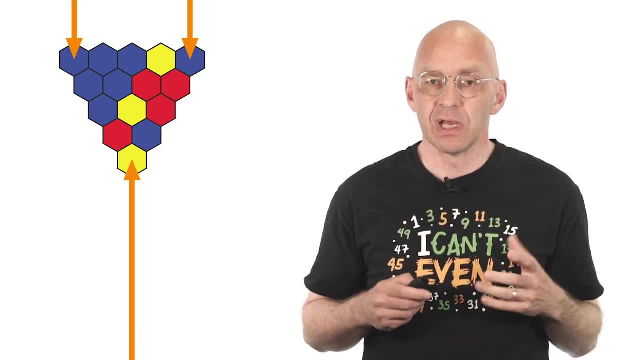 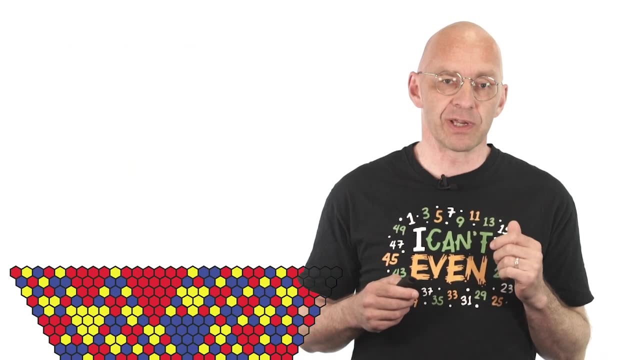 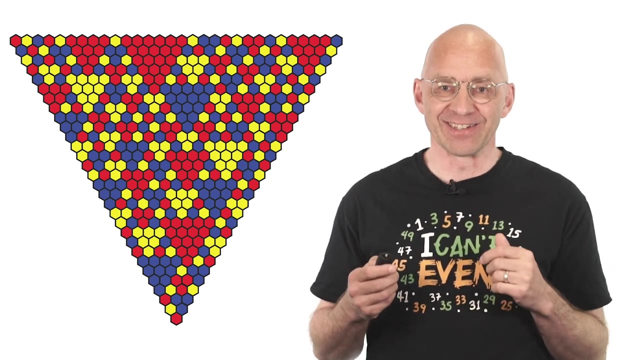 Okay, so why is 10 special, And are there any other special numbers? To hunt for clues, let's have a closer look at this larger triangle. Notice all the smaller solid-colored lines. here and there It's raining, little triangles, Yeah, raining, raining, raining. 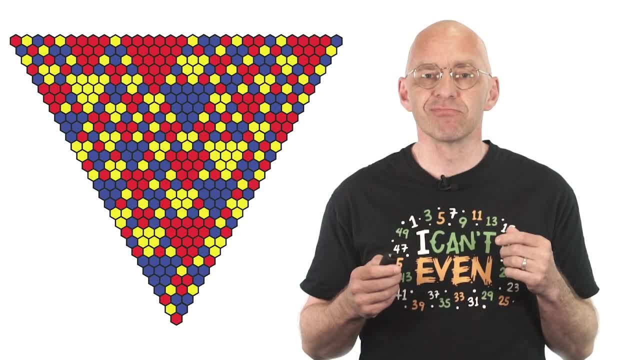 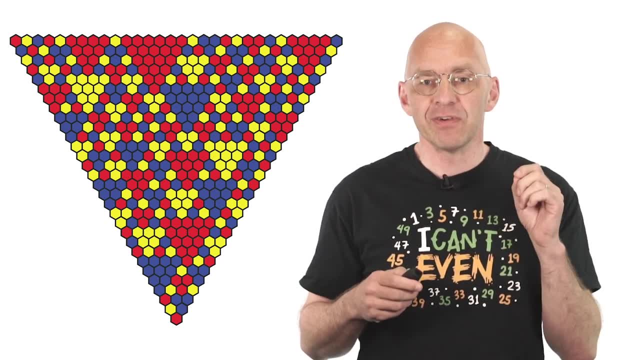 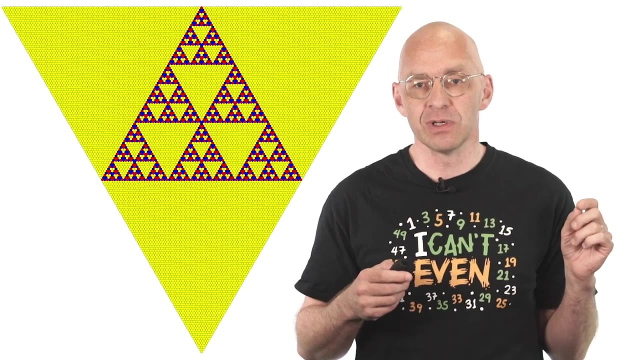 Maybe this reminds you of something. Hmm, Can you think of a famous mathematical supermodel dressed in little triangles? No, Okay, have a look at this special supersymmetric example. In this case, the first row is entirely yellow, except for a single red hexagon in the middle. 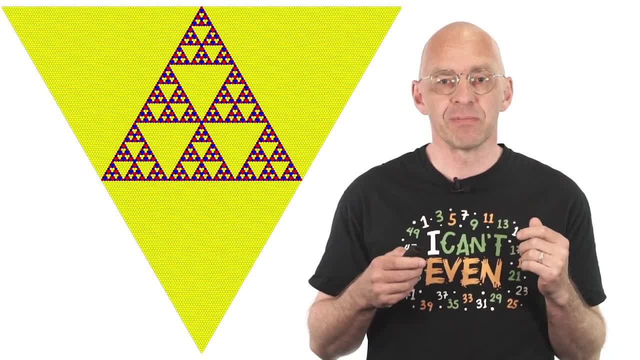 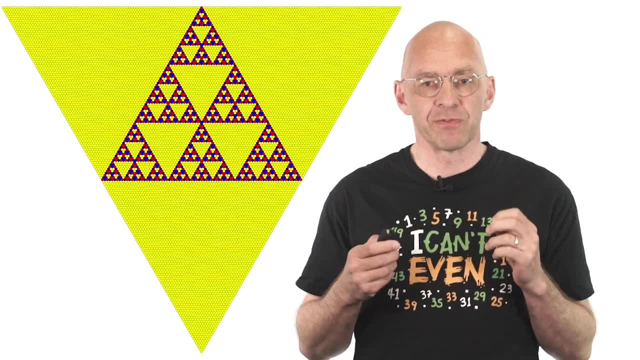 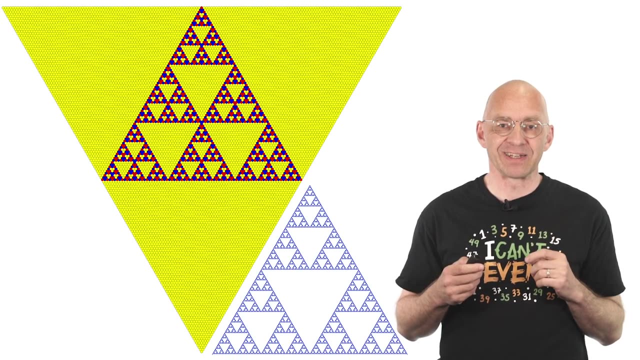 I first encountered a strange shortcut phenomenon in an article by mathematicians Erhard Behrens and Steve Humble in The Mathematical Intelligencer. It reminded me of the famous Sapinski triangle fractal, in which it is also raining little triangles. Beautiful pattern, isn't it? And I was also reminded of the pattern on a giant snail shell. 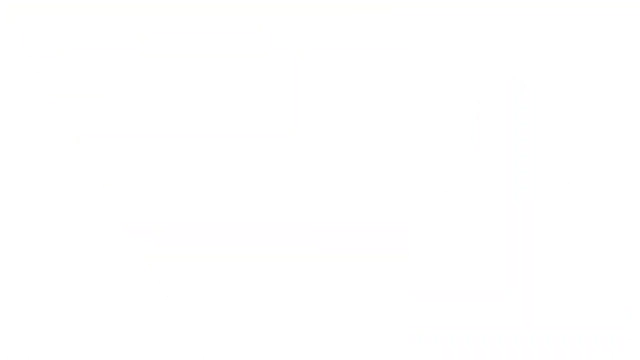 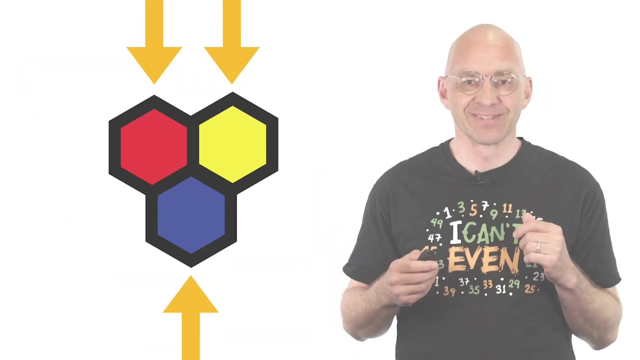 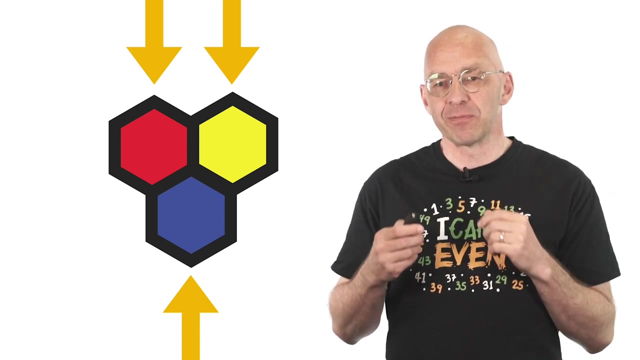 that I bought a couple of years ago in a butcher shop here in Melbourne- Butcher shop, Yep, you can find the strangest things in Australian butcher shops. And of course the whole summing two above gives the one below. business should be very, very familiar. 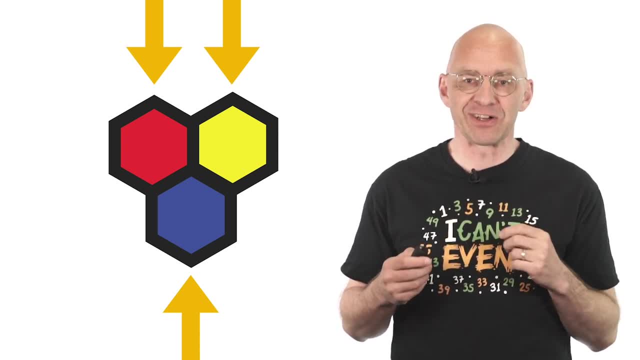 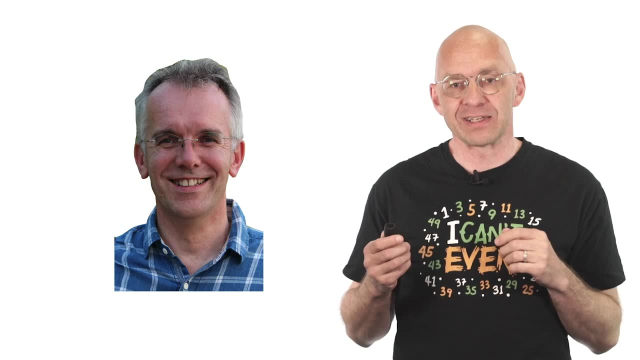 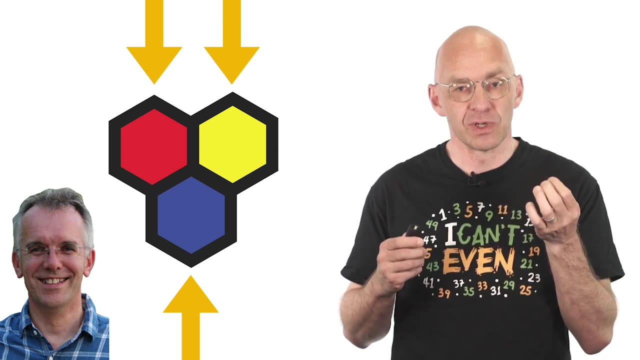 Yep, our good old friend Pascal's triangle is based on the same sort of growth principle. Steve Humble, one of the authors of the article I mentioned earlier, created the three-color game as a mathematical outreach activity in 2002 and discovered the shortcut while demonstrating it to kids. 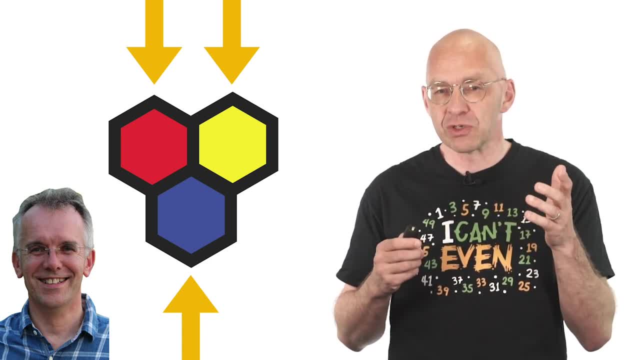 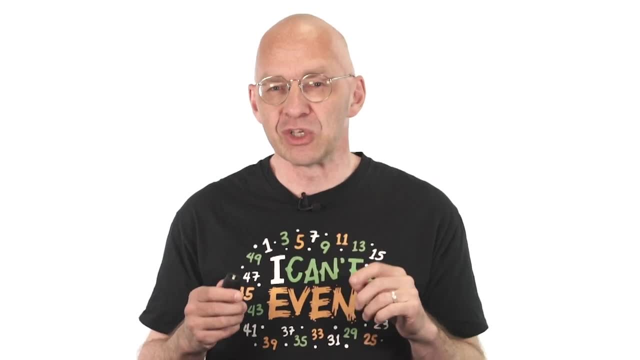 Today, I'd like you to imagine that you are a mathematician who, just like Steve, has stumbled across this mathematical gem. So, as a true mathematician, you are now cursed to not be able to sleep until you've come up with an explanation for. 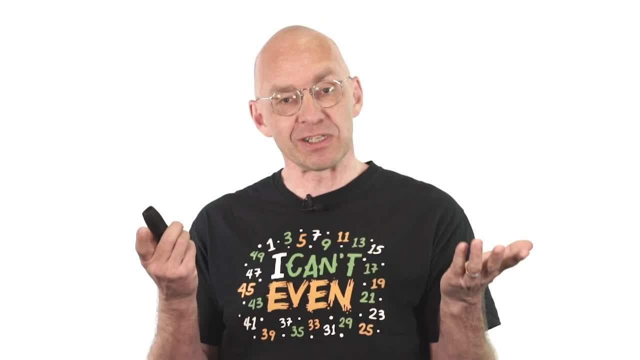 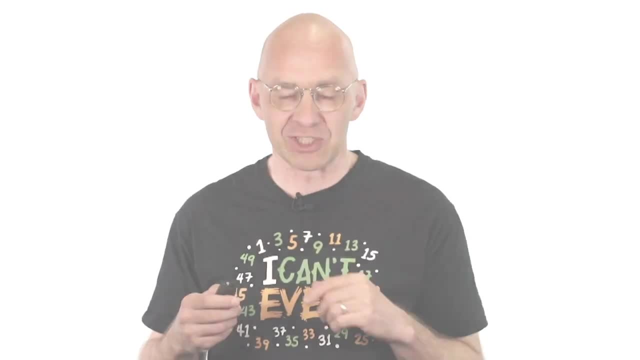 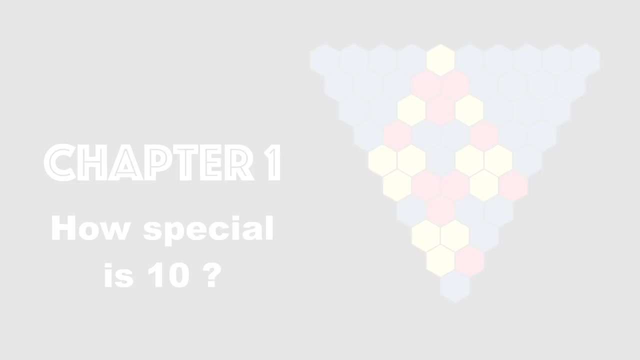 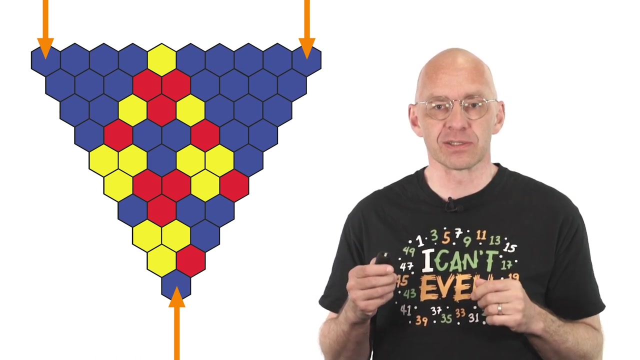 the shortcut and how it relates to the snail pattern and to Pascal's triangle and Sierpinski's triangle. Well, let's find out together, shall we? In five easy chapters. Okay time to investigate. Why does the shortcut work for Witt's ten triangles? 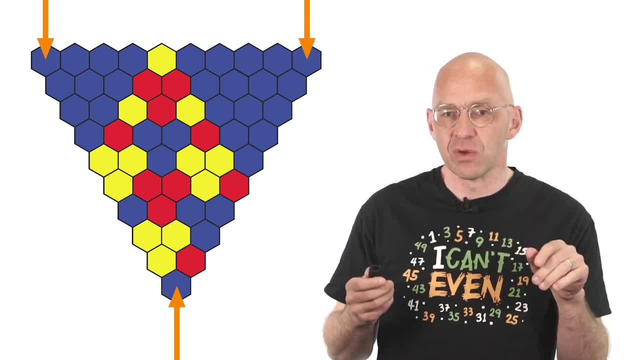 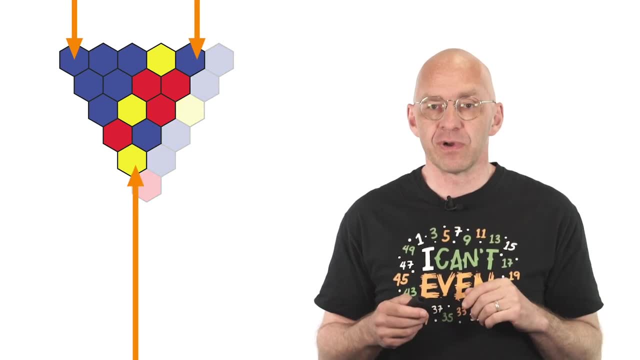 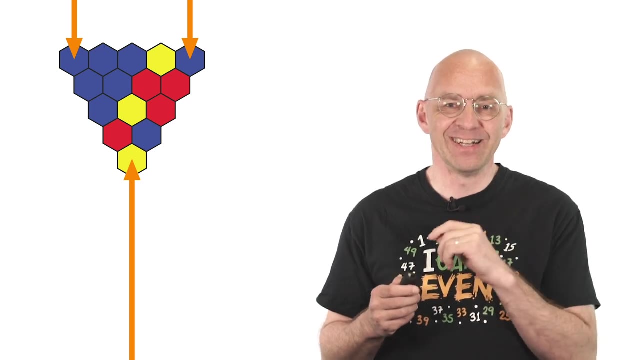 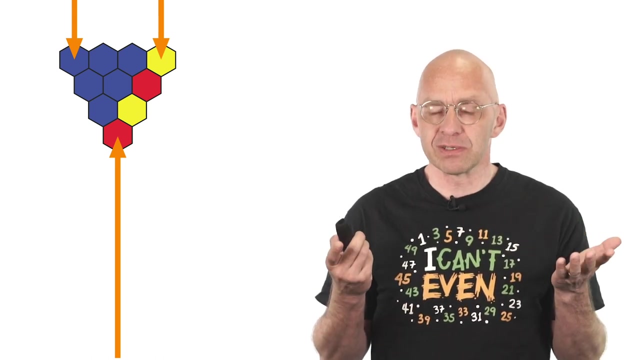 and are there any other special numbers? Well, we already saw that nine, eight, seven, six and five are not special, And that's where we stopped. Hmm, I wonder why. Okay, Let's have a look at 4.. Blue plus yellow is red. Probably also just a fluke, right? 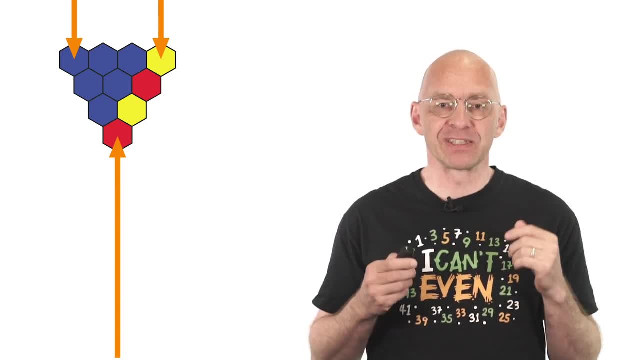 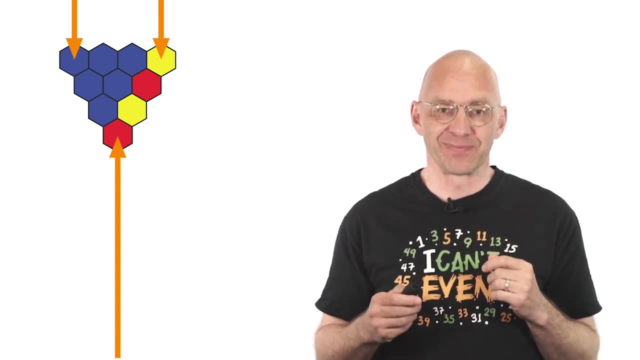 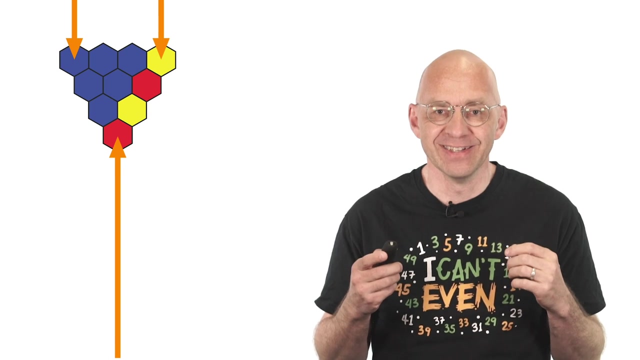 Wrong. If you keep experimenting with 4 triangles, you'll find that the shortcut always works. 4 is also special. Okay, let's say it's been a long night and we're all pretty brain-dead in this state. Can we still show that 4 is? 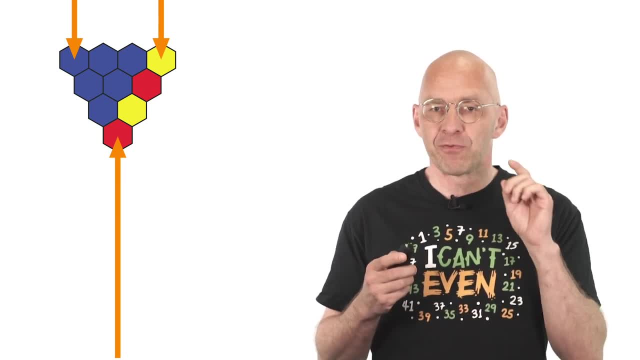 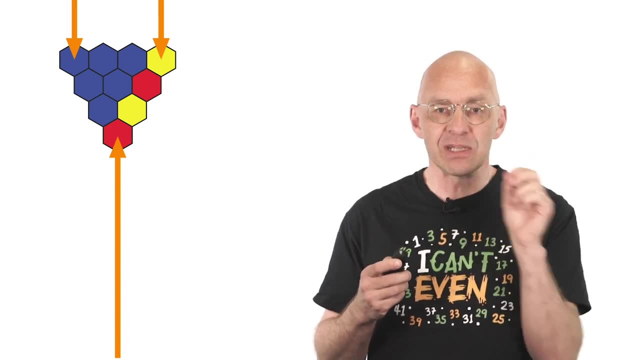 special? Yes, no problem. There are 4 hexagons in the first row and 3 possible colors. This translates into 3 to the power of 4.. That's 81 different ways to color the first row. This means that there are exactly 81 widths for. 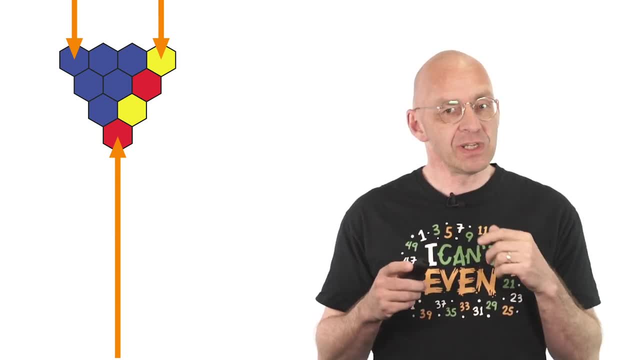 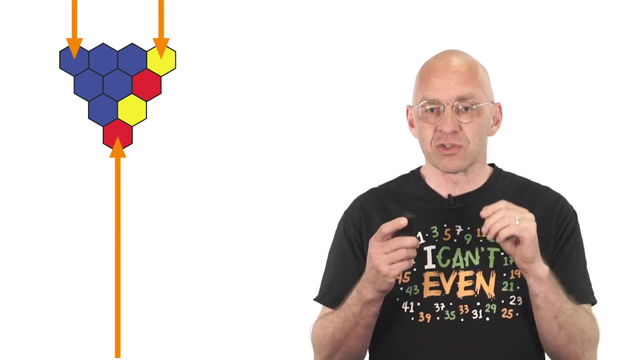 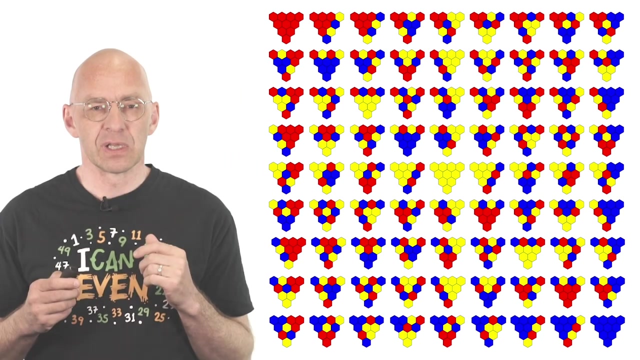 triangles, And even if I'm half dead, I can quickly throw together a computer program that will in an instant list all these triangles and check that our shortcut works- works for all of them. Actually, if we're not quite so brain-deaded, then we can use 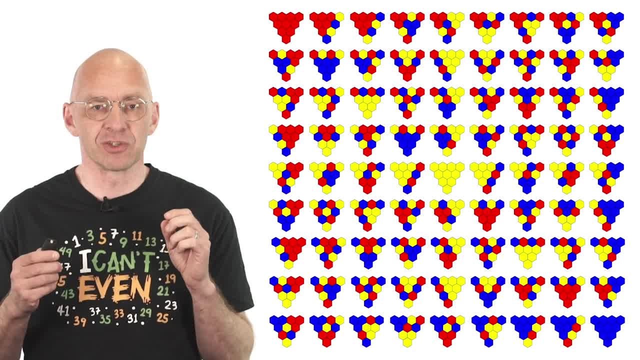 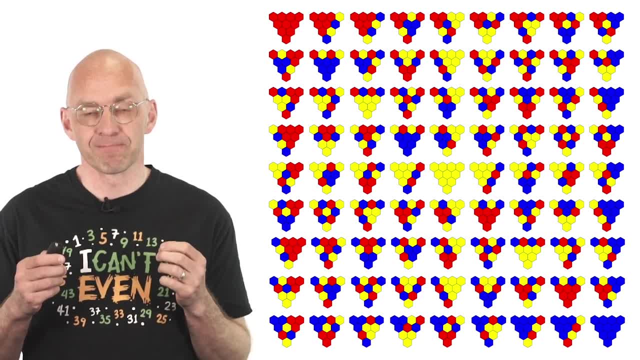 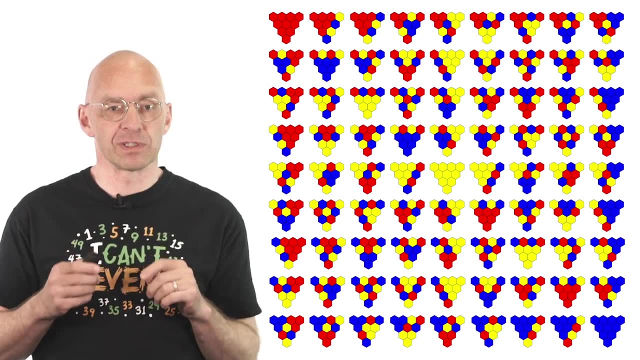 symmetry in permuting colors to reduce the number of triangles we need to check. So a little challenge for you: How many essentially different widths 4 triangles are there? Let us know in the comments. Of course, checking all those triangles doesn't tell us why 4 is special. We still haven't proved that 10 is special. 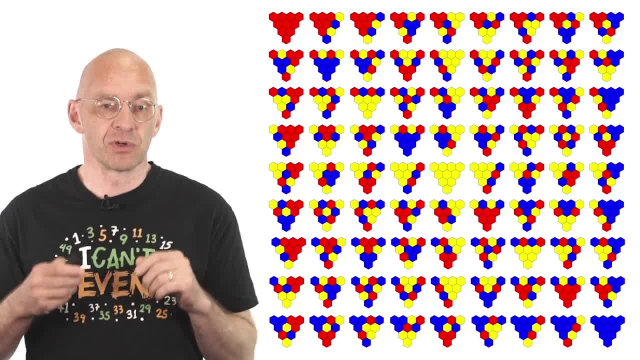 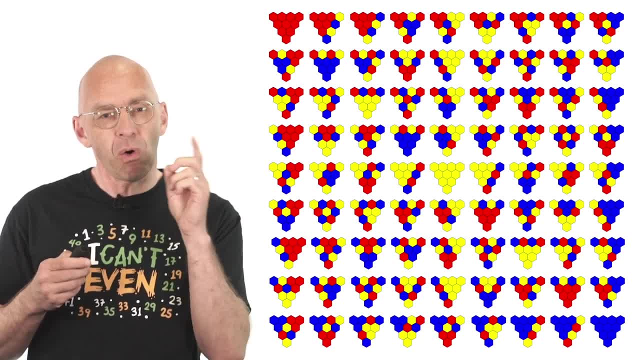 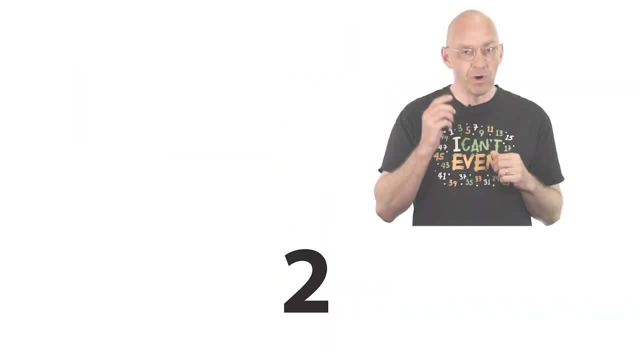 and we haven't checked many other widths. so it's time to go deeper. With my computer program I can also quickly make up larger width triangles and check that, among all the numbers from 1 to 100, the only numbers that appear to be special are 2, 4, 10, 28 and 82.. 2, 4, 10, 28,, 82. Tricky? Nope, not tricky at all. Did you see that time? Not that bad. 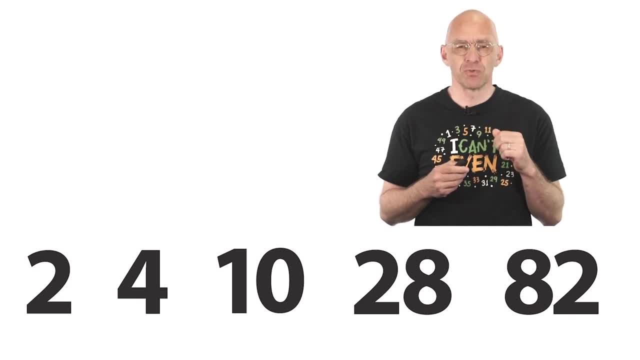 I hope you learned something today. See you next time. Bye, spot the pattern. These numbers are all 1 up from a power of 3.. 4, that's 3 plus 1.. 10, 3 squared plus 1.. 28,, 3 cubed plus 1. 82,, 3 to the power 4 plus 1.. And let's not 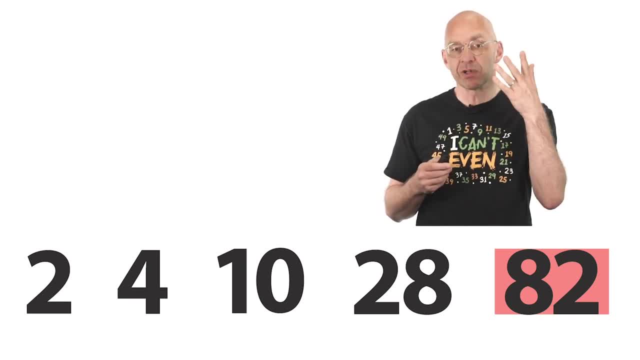 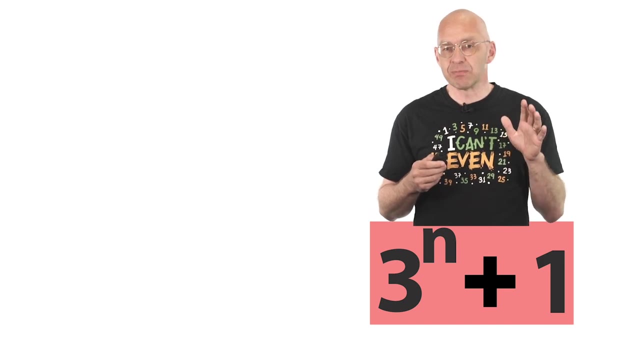 forget 2 at the beginning. 2 is 3 to the power of 0 plus 1.. The plot thickens And, based of what we've got so far, we conjecture that exactly the numbers 1 up from powers of 3 are special. Now let me show you something absolutely. 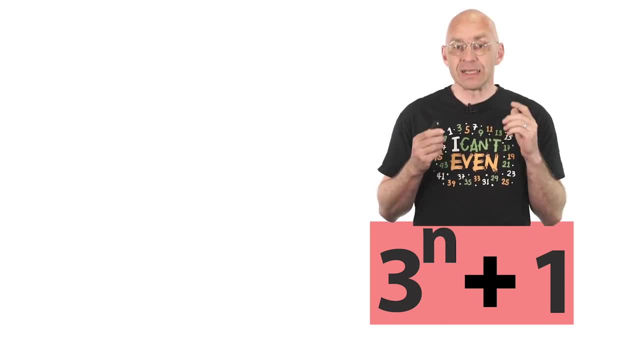 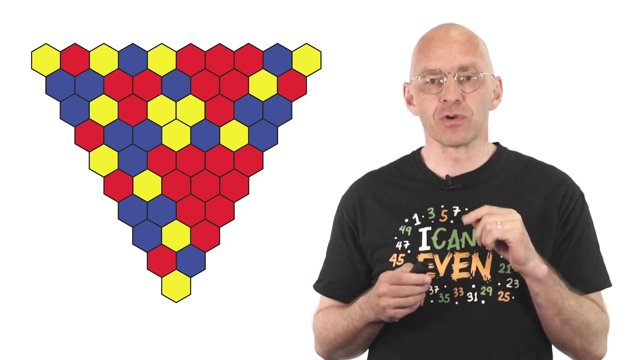 beautiful, A proof that all these numbers are indeed special. This one is really good promise. Let's begin where we began, by showing which 10 is special. So let's start with any old width 10 triangle. Now, if focus on these hexagons here, Then these three hexagons are the corners of this. 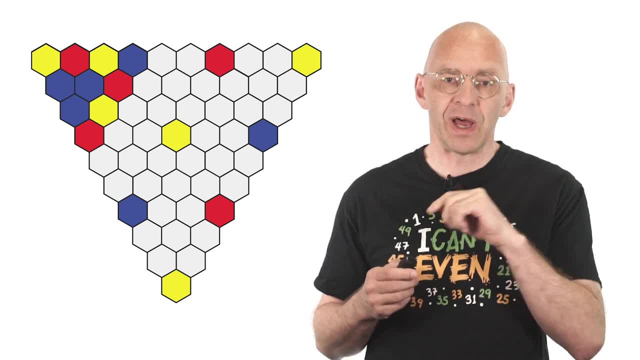 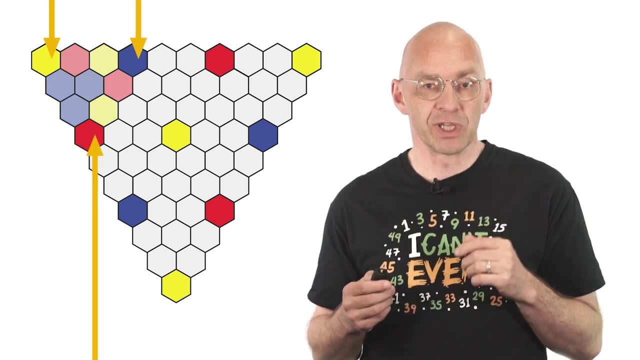 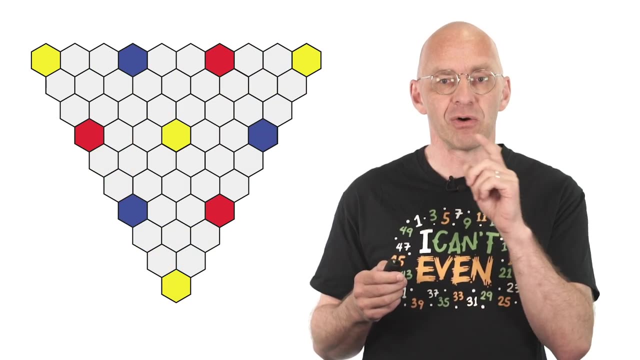 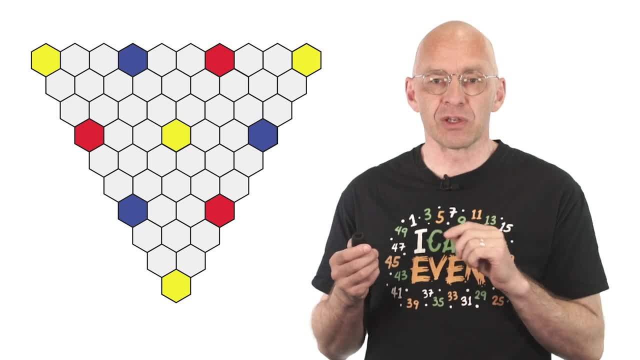 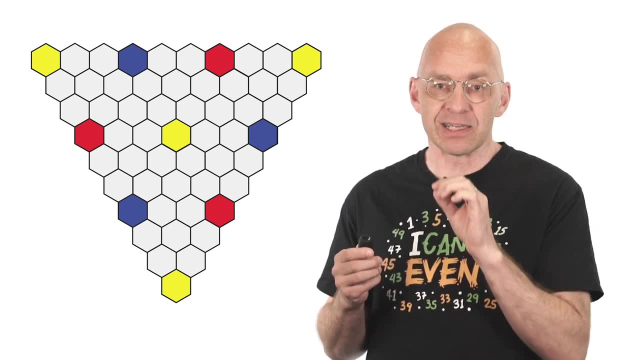 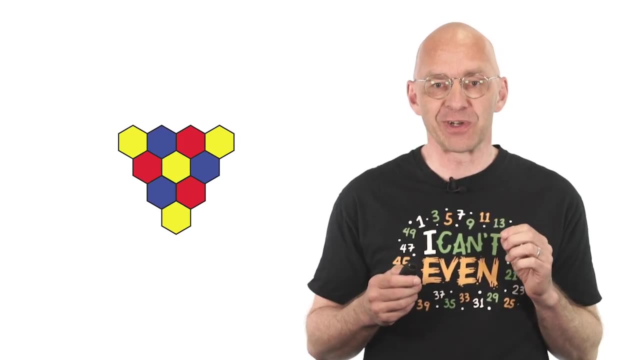 right. Can you see what's happening? We just showed that over there. any two adjacent colors add to the color below, And what this means is that these highlighted hexagons combine into a width 4 triangle And therefore, because 4 is special, the top two corners add to the. 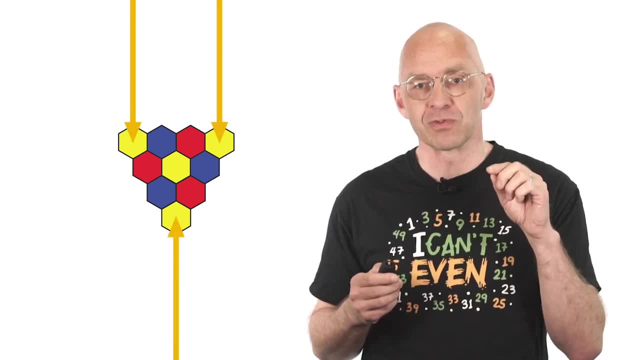 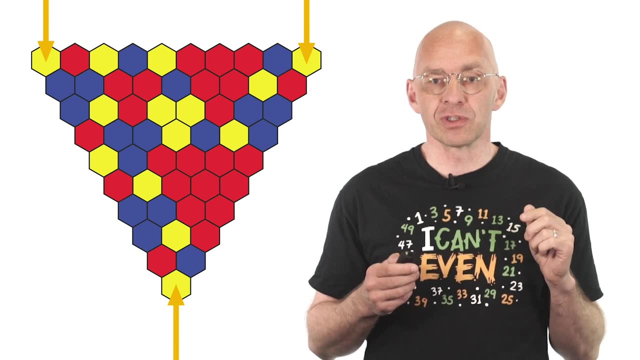 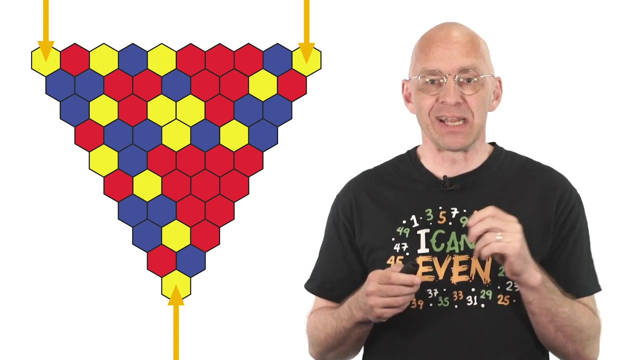 bottom corner. But since the top corners of this width 4 triangles are also the top corners of the original width 10 triangle, it follows that the top two corners of a width 10 triangle add to the bottom corner Always. In other words, 10 is special. An argument like this makes my day So on. 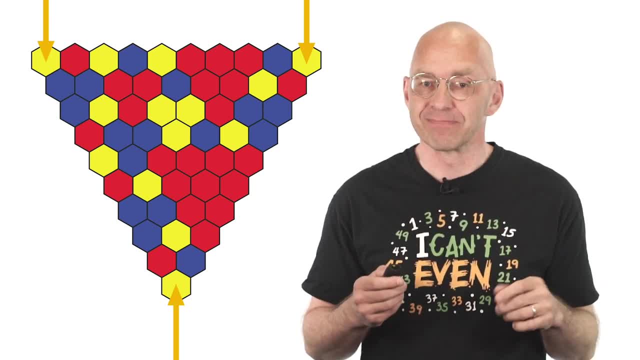 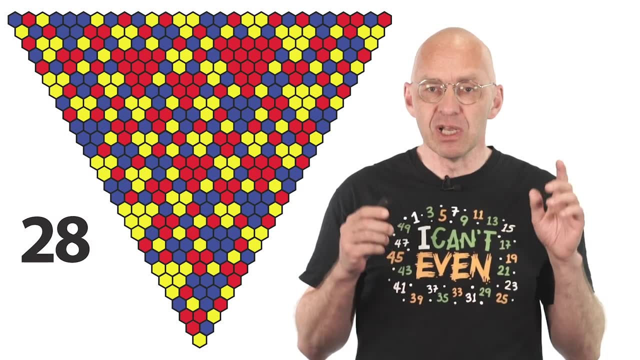 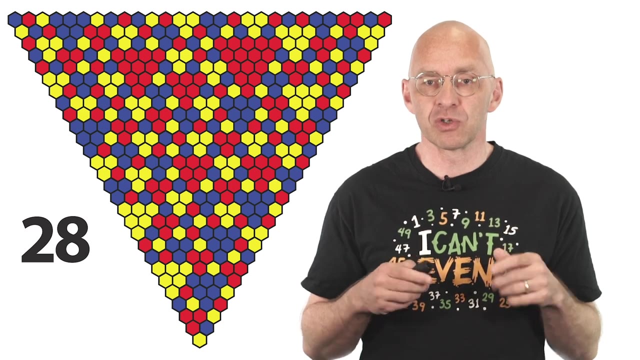 the scale from 1 to 10. how beautiful an argument is this? Yep, we're doing polling now. Let me know in the comments what you think To prove that 28 and indeed all the other powers of 3 plus 1 are special. we just repeat this argument over and. 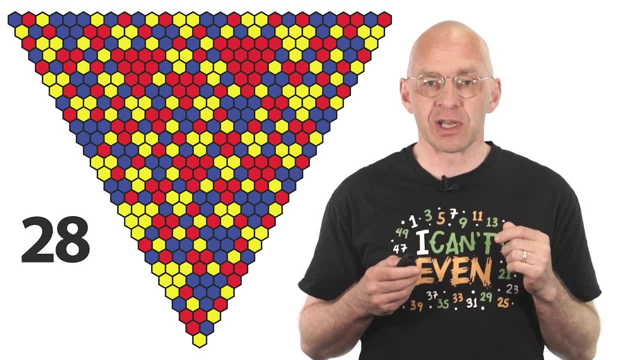 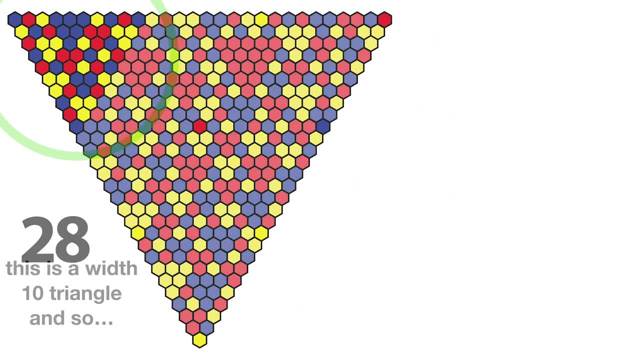 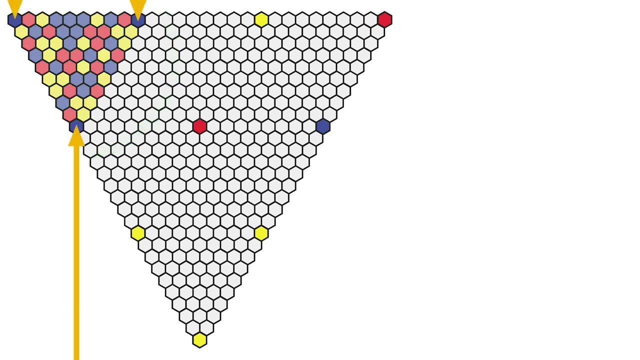 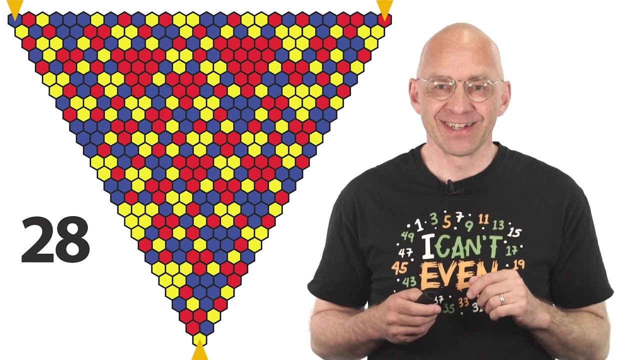 over Here does the question come up? Quick, animated. first iteration of the argument that shows that 28 is special using the fact that 4 and 10 are special. So nice And a little challenge for you. Can you think of a second way to argue? Hint switch. 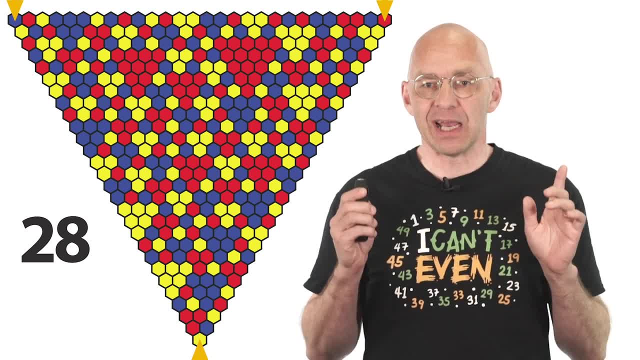 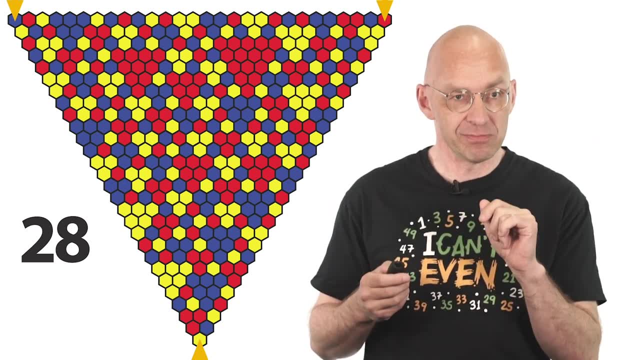 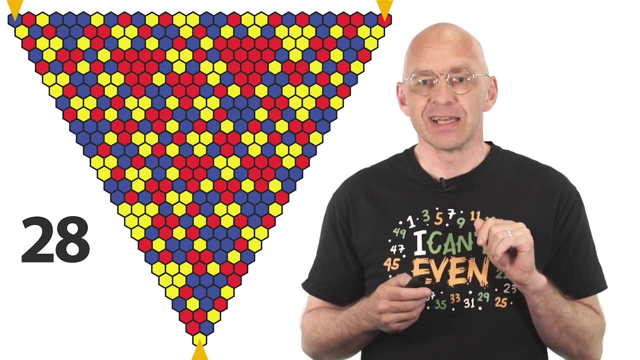 the roles played by 4 and 10.. Anyway, I suspect that at this point most people would declare the mystery solved, Time for a cat video. Well, that's not what we do here on Mathologer, right? Is it really just a big coincidence that width 4 is? 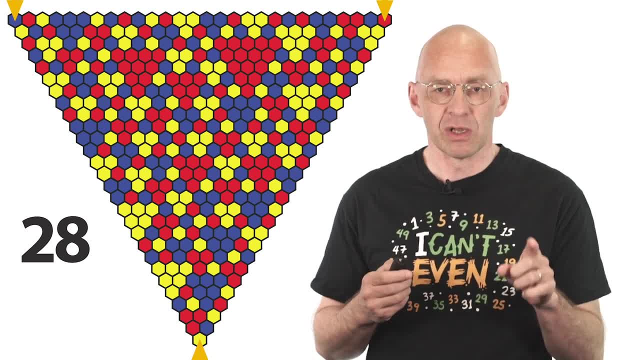 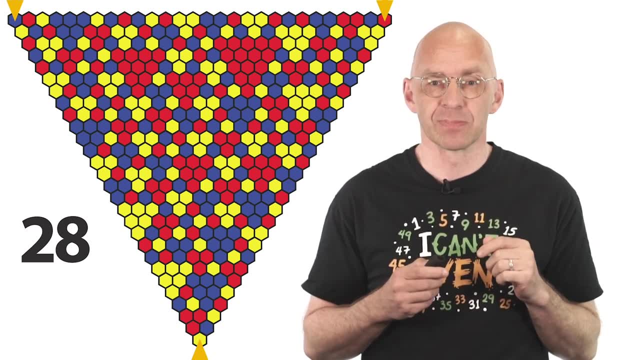 special or is there a deeper reason? Also, we know that 2,, 4,, 10, etc. are special and we suspect there are no others. But how can we be certain? And what's up with all these similar phenomena, Sapinski and the snail shells and what not? 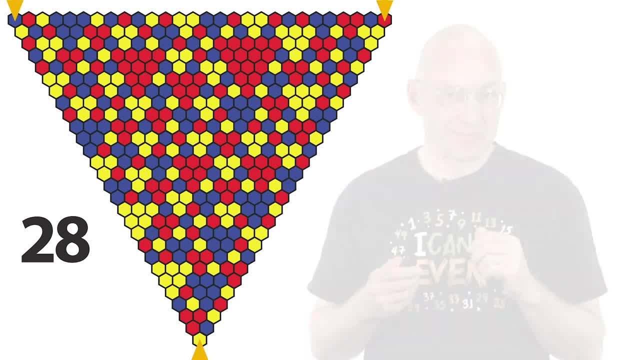 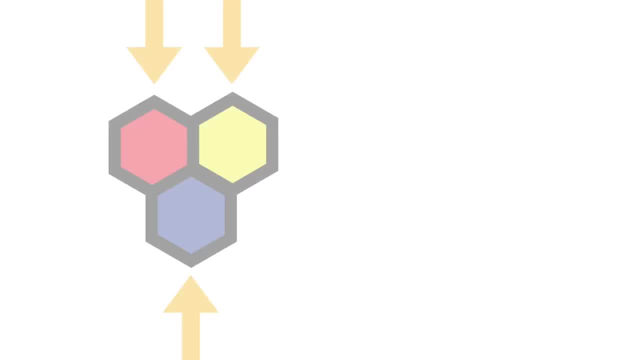 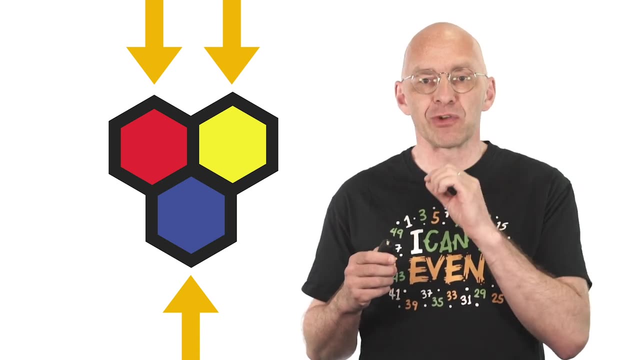 Are there any beautiful connections? Ready to go deeper? The basic rule of two adjacent colours in one row, summing to give the colour immediately underneath, just cries out for us to have a look at the tip of Pascal's triangle Right. Any two numbers in this famous 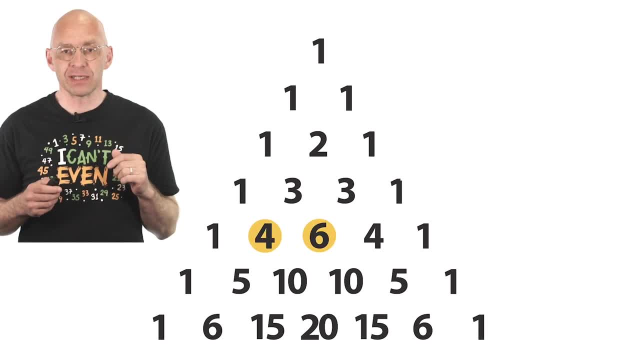 numbered triangle. add to the number right below here: 4 plus 6, that's 10.. 5 plus 1, that's 6.. Ok, This addition process is very similar to our colouring scheme, but there are also obvious differences. In Pascal's triangle there are no hexagons. We are adding. 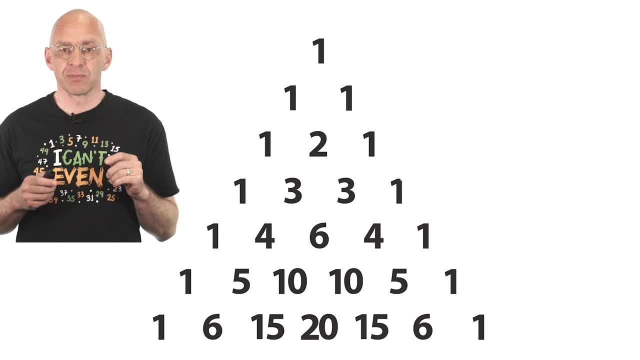 numbers instead of colours, And everything starts from the top of the number triangle. Everything starts from the tip rather than from a row of numbers. Hmmm, Ok, You want hexagons? Well, here are a couple. What else You want? the whole thing? 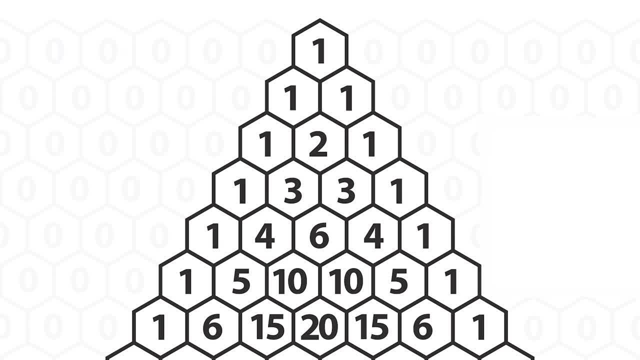 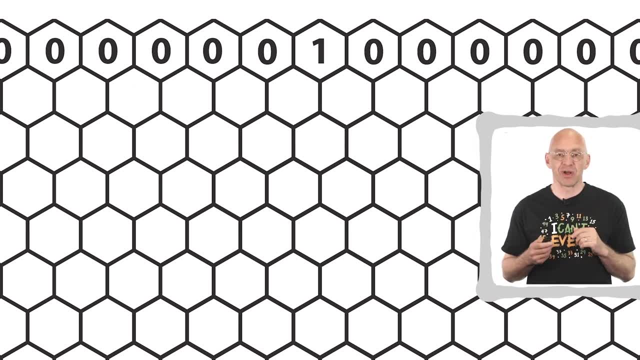 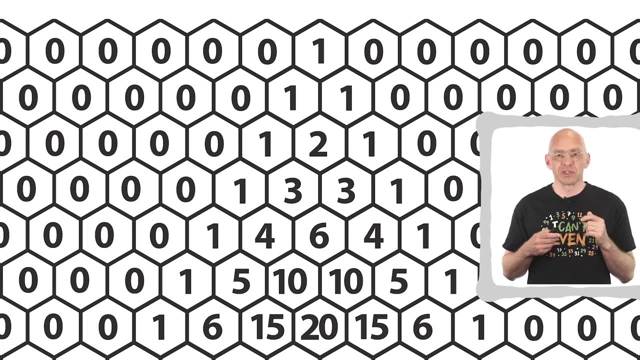 to start from a row, not from the tip, Not a problem at all. So we can think of Pascal's triangle growing from an infinite row of zeros, with a single one thrown in somewhere in the middle. And that should also remind you of the Sapinski-ish coloured triangle we saw. 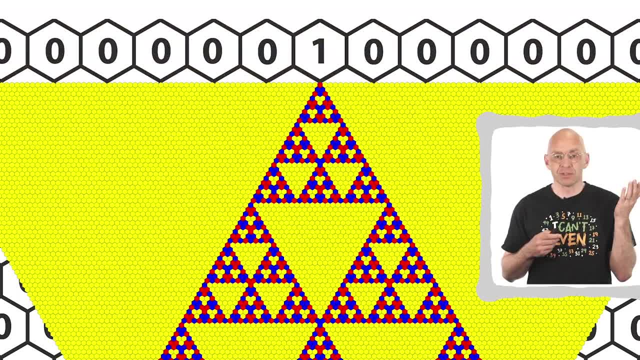 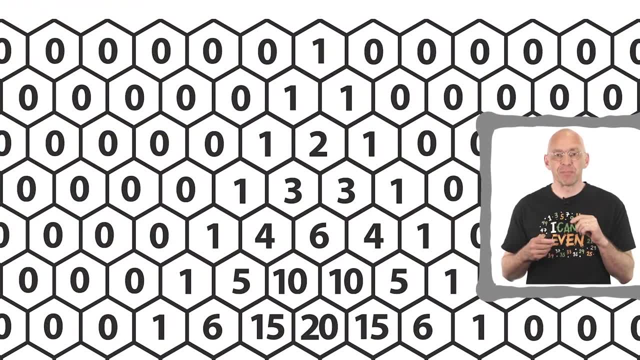 earlier, Which starts from a row of yellows with one red exception in the middle. Interesting huh. Anyway, to keep things uncluttered and to escape from this frame here, I'll hide all the zeros anyway, and we'll return to the familiar picture of Pascal's triangle. Ok, 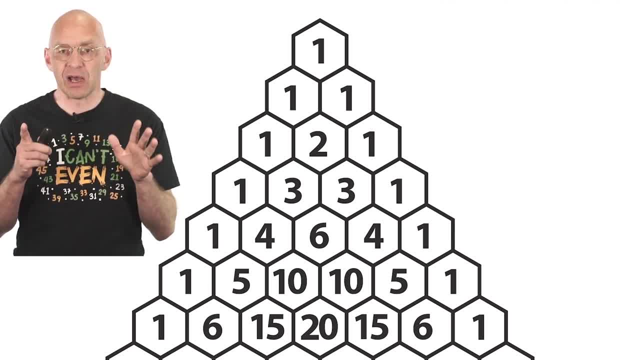 Just remember that the zeros are still there, but hidden. Now, what about colours? Well, the first idea that comes to mind is to colour the hexagons according to one of the natural ways to split the integers into a finite number of classes, For example, colouring all the odd numbers dark and the even numbers. 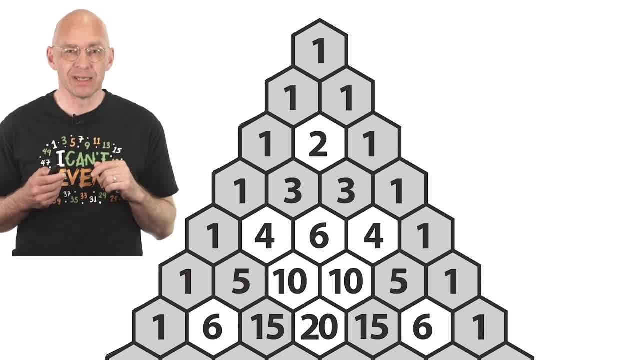 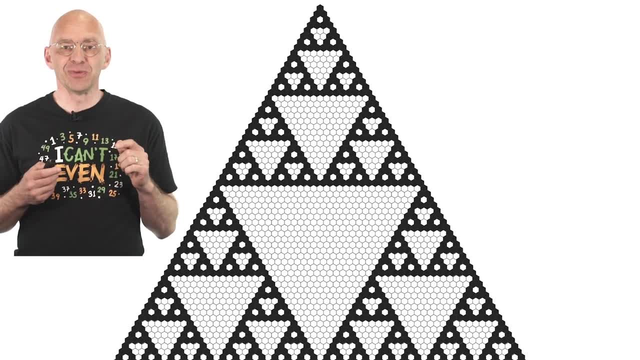 white. we get this. That looks promising. And it's even more promising when we zoom out to reveal a larger slice of our triangle. Wooh, pretty impressive, huh? In fact, if you keep zooming out, our ever more detailed, even odd triangles will converge to the famous 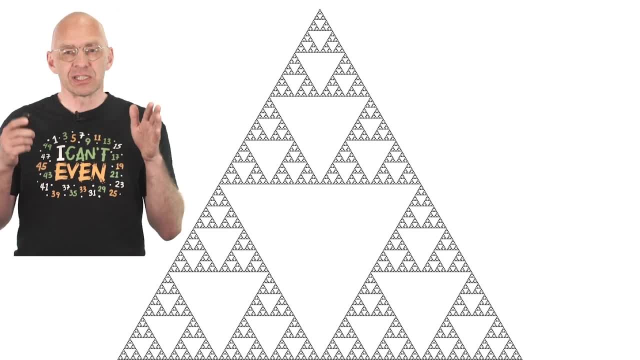 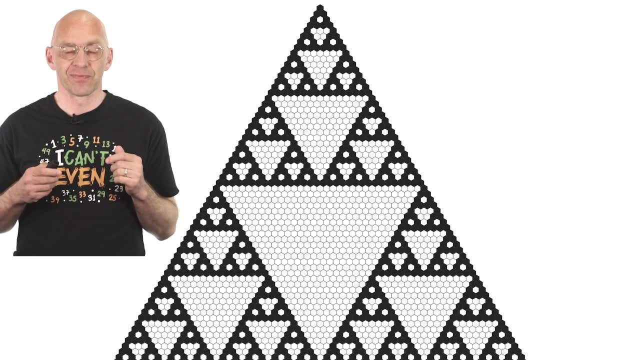 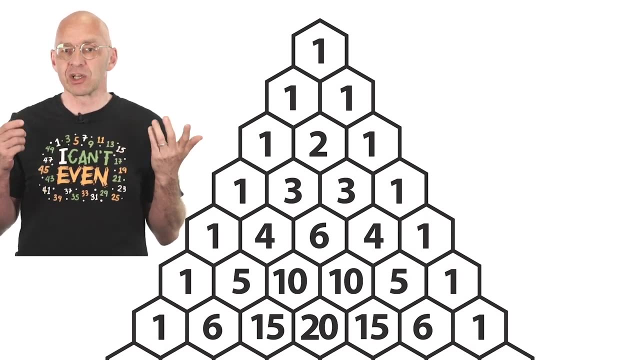 Sapinski Triangle, Fractal. Anyway, it's most definitely raining little triangles in there, just like in our 3 coloured triangles. Another way to interpret our odd even colouring is to say that we colour according to what remainder a number has on division by 2.. After division: 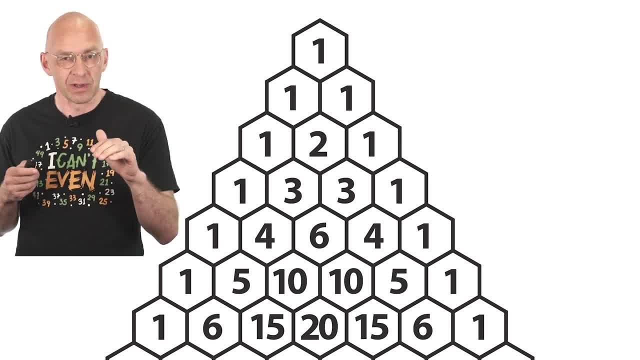 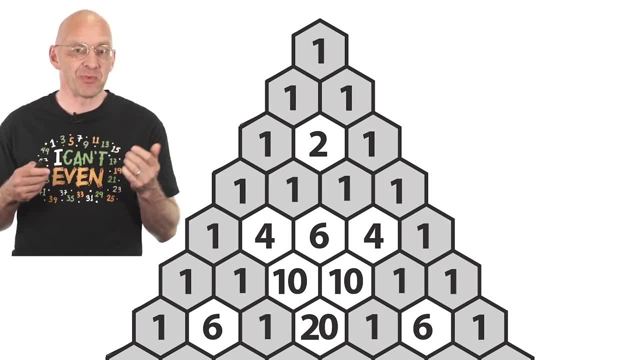 by 2, the possible remainders are 0 and 1.. For odd numbers, the remainder is 1 and we color dark. For even numbers, the remainder is 0 and we color in white. What we then get is Pascal's triangle using what is called base two modular. 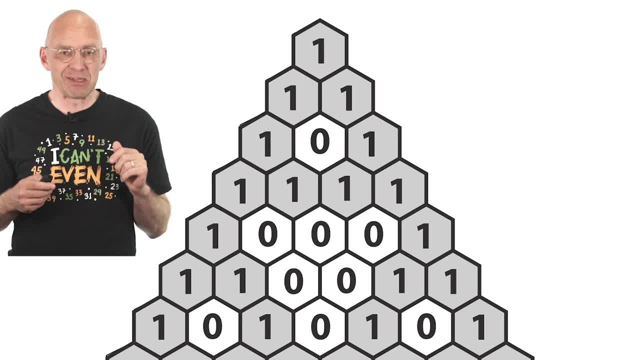 arithmetic Fancy words, but it's just even and odd. So wherever you see 1 and 0 next to each other, there will be a 1 underneath. 0 plus 1 equals 1.. That translates to even plus odd equals odd. Similarly, 0 plus 0 equals 0.. And then 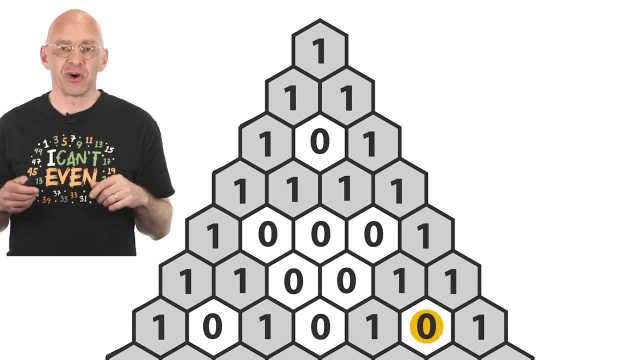 there's the slightly weird: 1 plus 1 equals 0, which amounts to odd plus odd equals even. Okay, we found a natural numberish way of coloring with two different colors. What happens now if we play our game with the even odd rule Are? 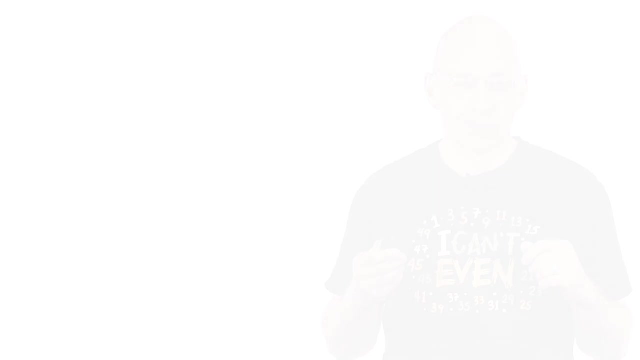 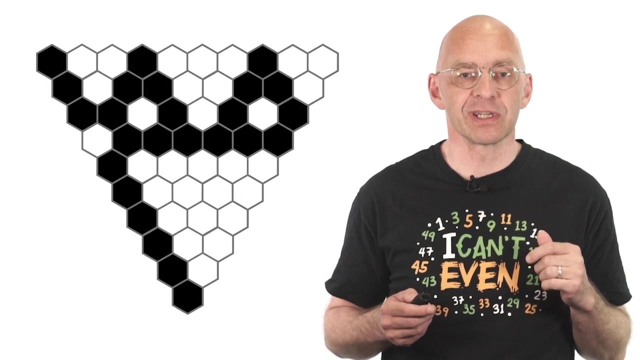 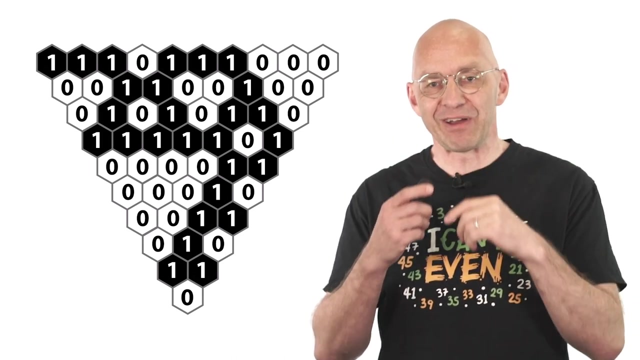 widths: 10 triangles still special? Hmm, here a few random widths: 10 triangles. you get this way: There's 1, there's another 1, there's another one, there's another 1, another 1, and well, is 10 still special? No, definitely not, If it were black and 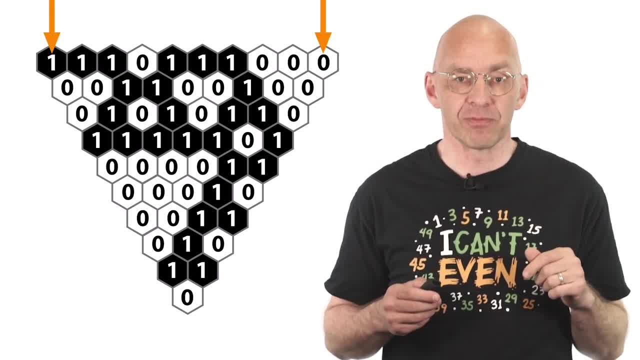 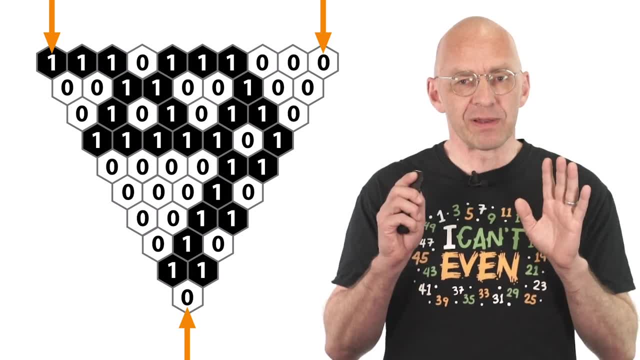 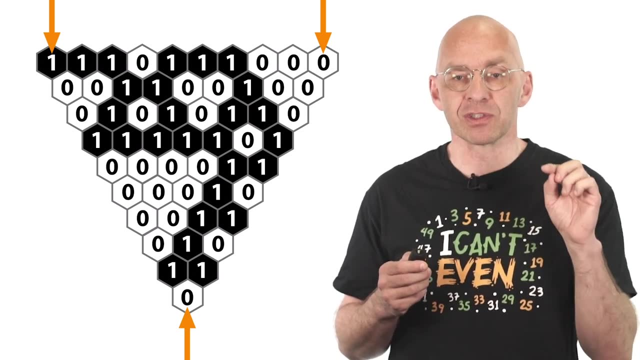 white on top should give black at the bottom right. 1 plus 0 equals 1.. Not 0.. we got it right at the bottom, But don't despair, There are also special widths for our even odd coloring. However, instead of 1 plus powers of. 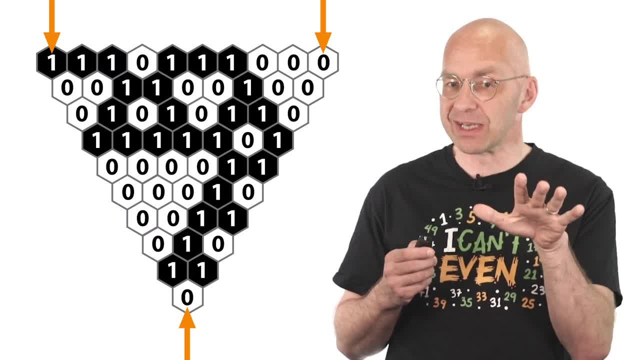 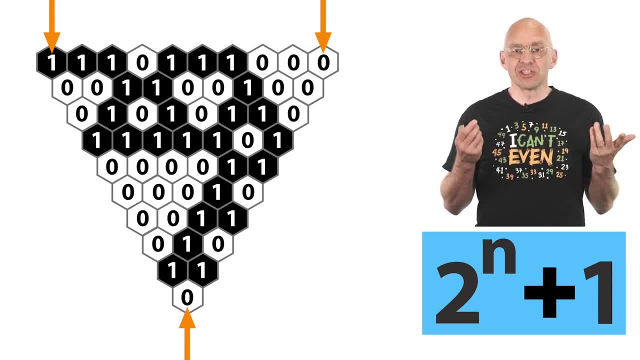 3,. this time it's 1 plus, can you guess it- powers of 2.. It is easy to prove that all these numbers are special using the same collapsing argument as for our red, yellow, blue triangles. This lovely and simple construction also suggests a very 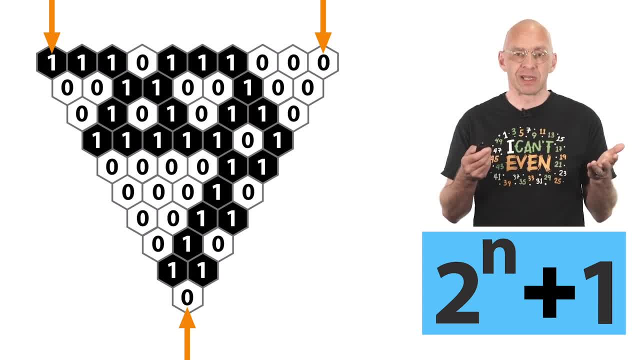 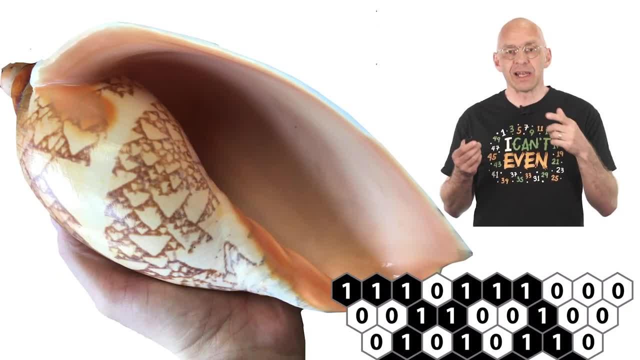 natural model that can be used to at least partly explain the formation of snail shell patterns. A snail shell grows in thin layers that are added onto its lip. In our mathematical model, these layers are the horizontal rows of hexagons. Then the color of the hexagons in each new layer is determined by the 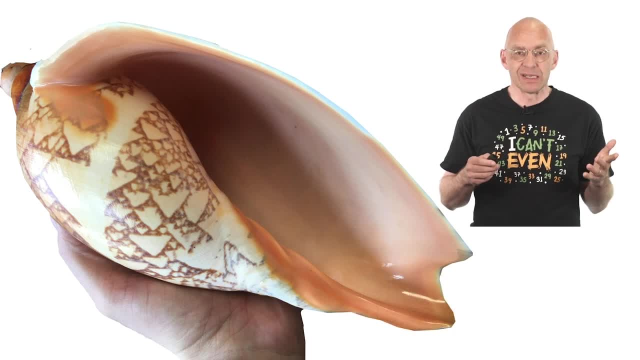 simple rules for adding odd and even numbers. This is all very neat, and it is based upon a biological mechanism that can be observed, where the characteristics of existing cells are determined by the color of the hexagons. So nature has already found a lovely application of the games we are playing. 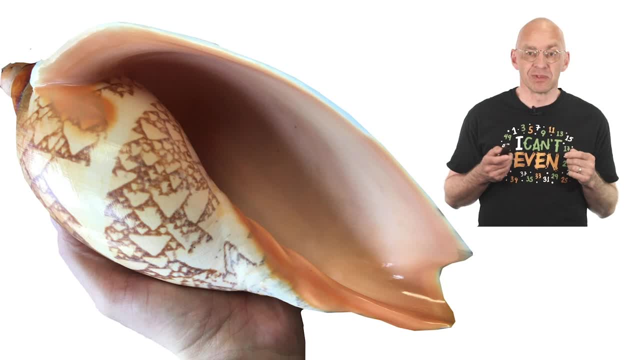 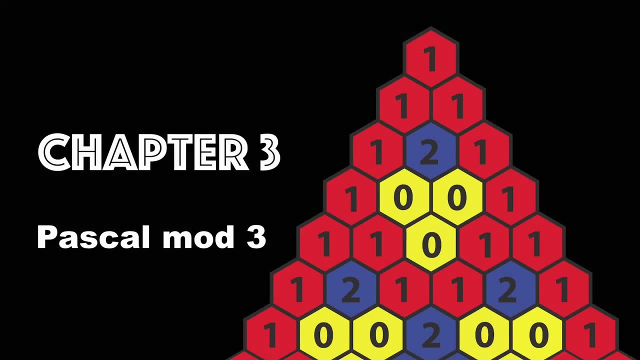 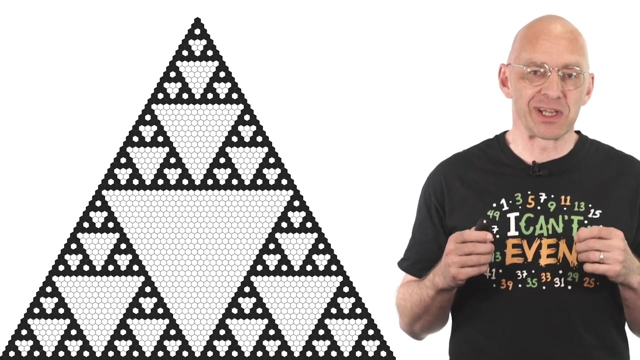 here. Do any of you apply similar this, plus that mathematics, in anything you do in your working life? Let us know in the comments. Okay, so this is what Pascal's triangle looks like when you color it according to the rule of law. If you want to learn more about it, please subscribe to our channel. 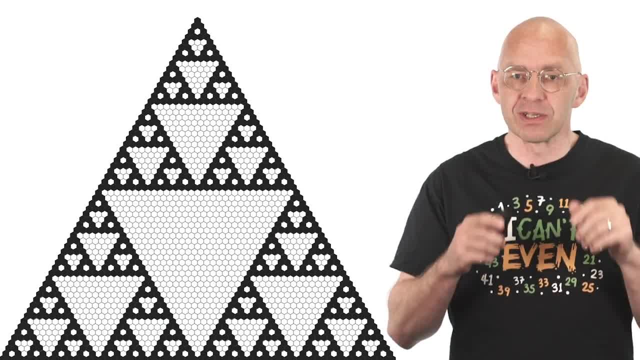 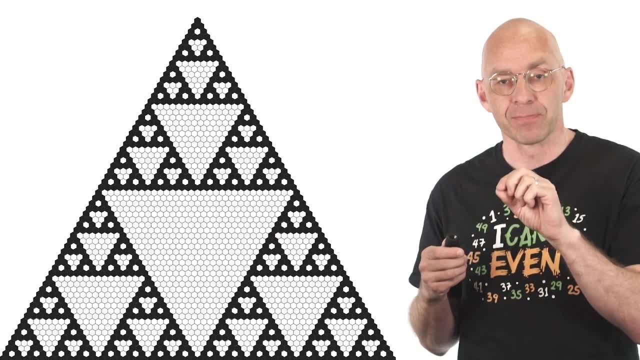 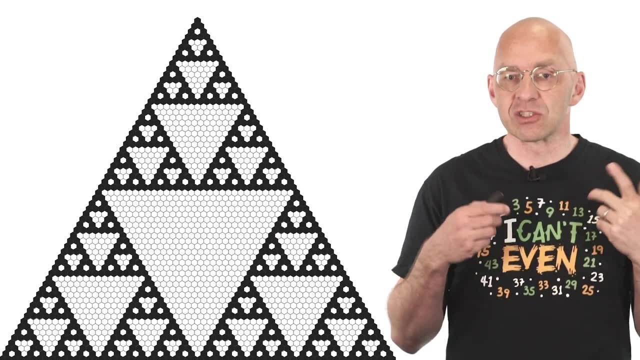 For our original game we used three colors, so let's see what happens when we use remainder on division by three. Of course. now the possible remainders are 0,, 1 and 2, and let's respectively assign them the colors yellow, red and blue. Then 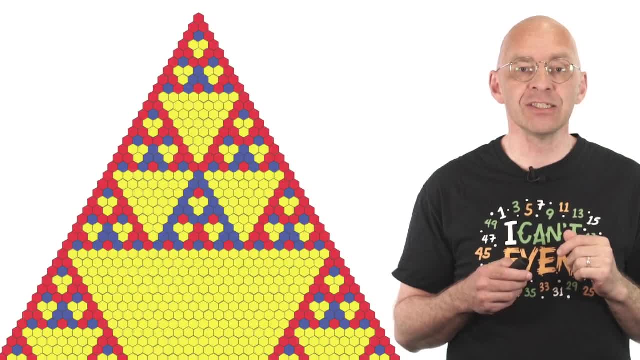 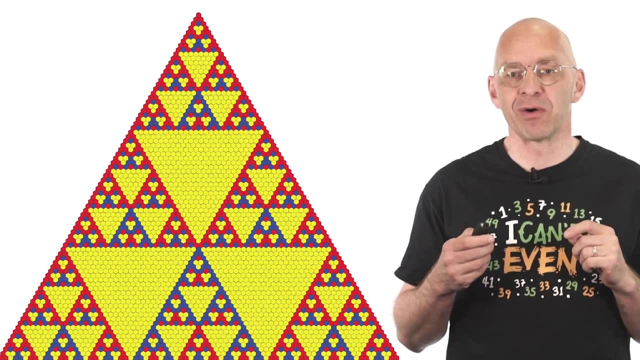 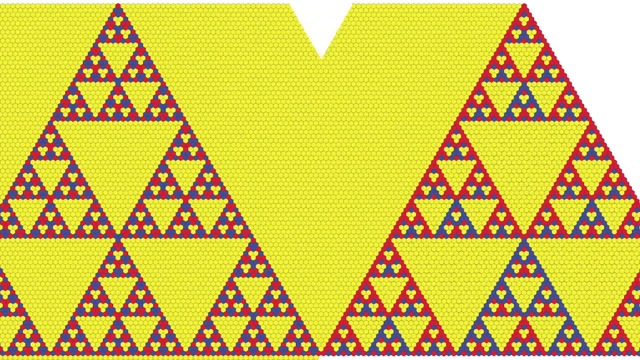 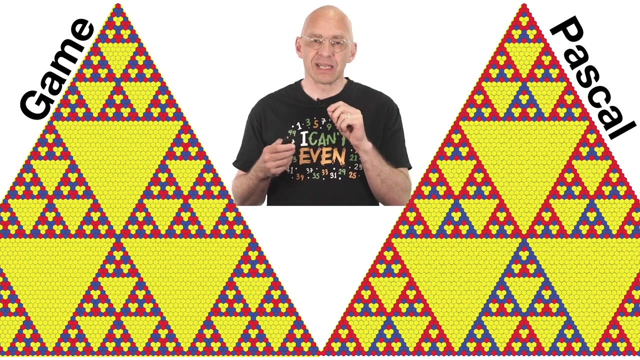 this is what you get. Very pretty again. Now compare this triangle to the nicely symmetric triangle that resulted from our original three color game. Yep, so close, Not quite the same, but we're definitely on to something. Okay, let's have a close look at the growth rules for our remainder three: Pascal. 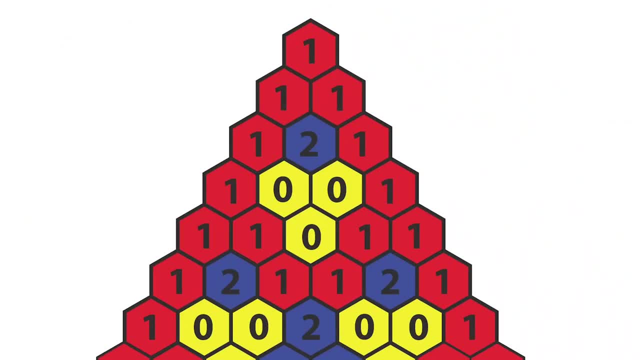 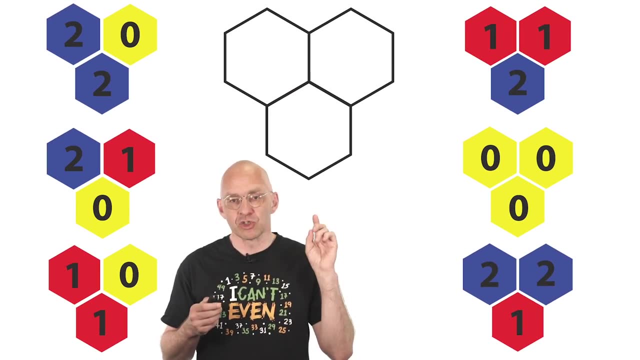 triangle. So with Pascal to add a and b, we simply go a plus b, mod 3.. Now, in terms of colors, this doesn't quite correspond to what happens in our original color game. For example, in our original color game, red plus red equals red, But Pascal gives the. 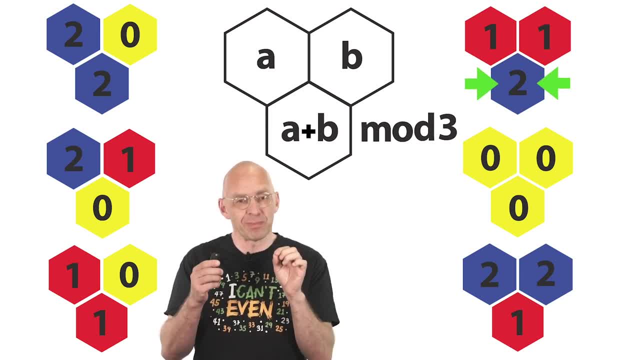 answer as blue. However, there's a super simple algebraic Eljebric adjustment to get perfect agreement. Can you see what we need to do? Well, first notice that at least the middle rules always work. But to make things work completely, these twos need to be replaced by ones, and these ones need to be replaced by. 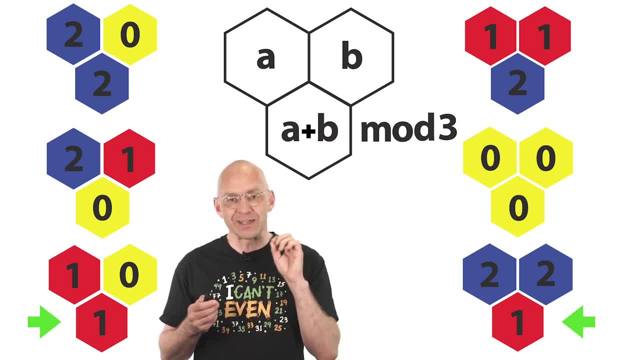 twos, And there's a really simple tweak to do that. Just go minus a, plus b here. Let's check that this tweak really has the desired effect. Okay, minus zero. well, it's zero. nothing changes here, which is great. What about the top rules? Well, now, 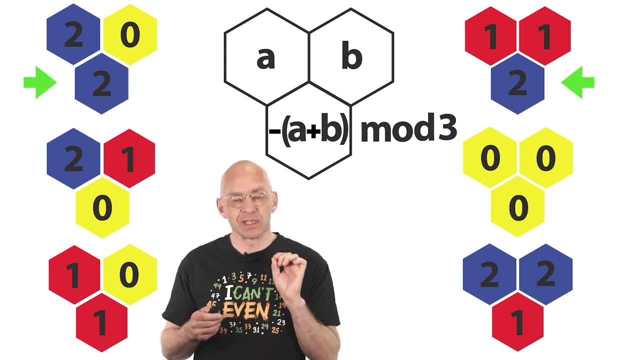 we have minus two, but in mod three arithmetic minus two is the same as minus two plus three, which equals one. Got it. And on the bottom row we now get minus one, which is equal to minus one plus three equals two. This really works. 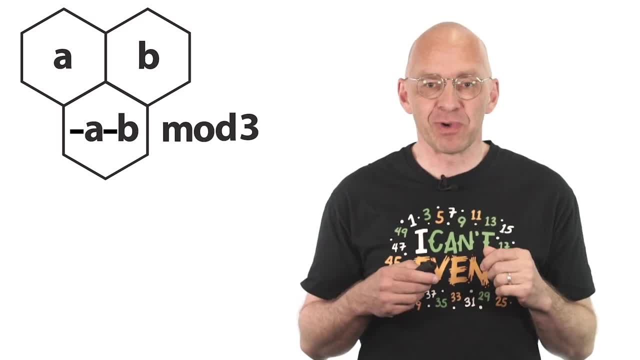 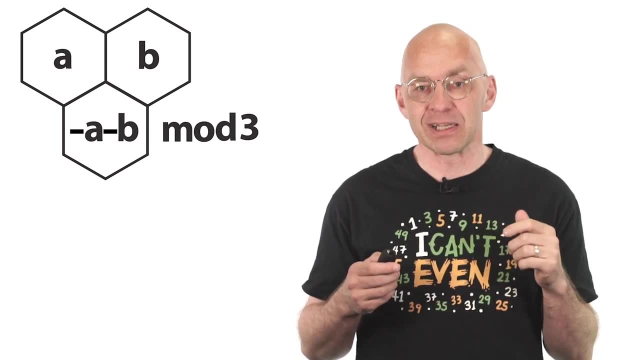 Let's do it again. So we've done it. This algebraic rule has captured the mathematical soul of our original three color game. As a first application of this clever insight, let me show you how you can see pretty much at a glance why four was special in the 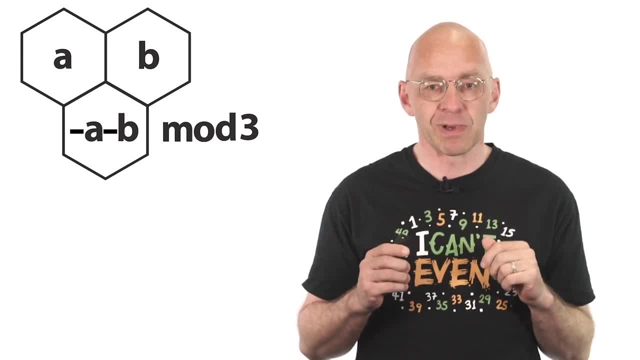 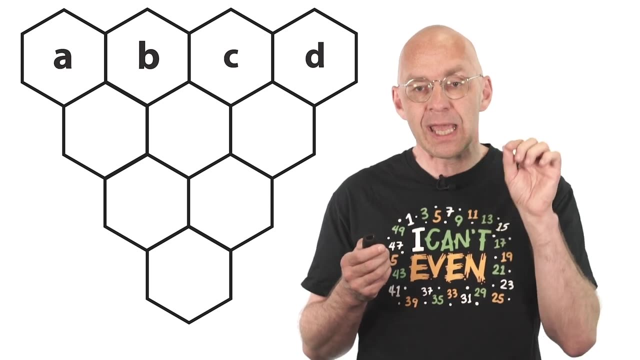 original game. Remember, originally we showed this by listing all possible 81 widths, four triangles and checking that the shortcut works for all of them. We can do much better than that using just a little algebra. We start with four random colors- a, b, c, d- and then we can simply calculate. 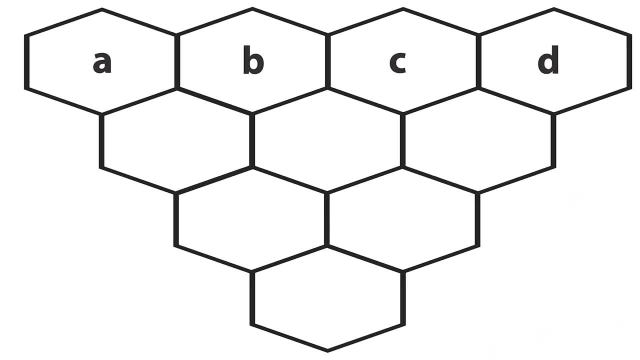 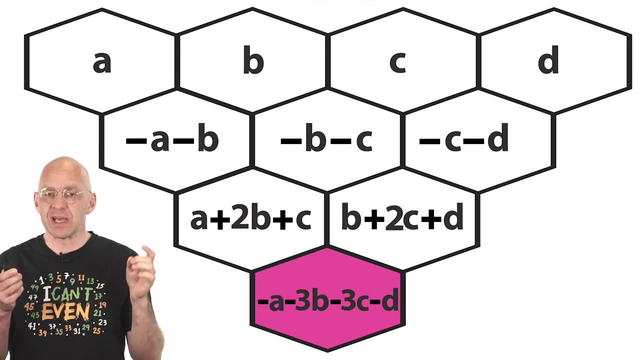 the remaining colors like this, But of course, in mod three, arithmetic three times, anything is just the same as zero. And so, hmm, fantastic, B and C just cancel out, and the number at the bottom only depends upon the numbers a and d in the top corners in the right way. So our simple calculation confirms once again. 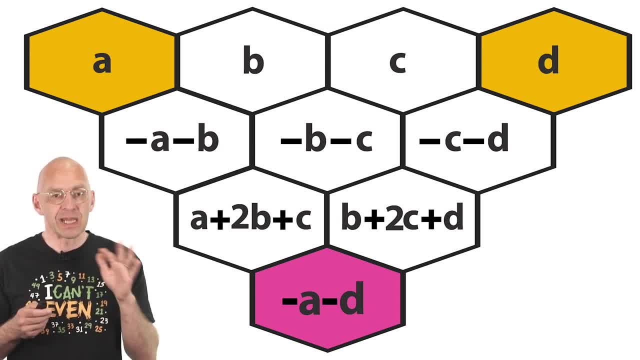 that four is special for our original setup. But actually this calculation tells us something about Pascal's triangle as well. Instead of our original three color game, take a look at the Pascal three color game. Then the algebra is exactly the same, except all the minuses. 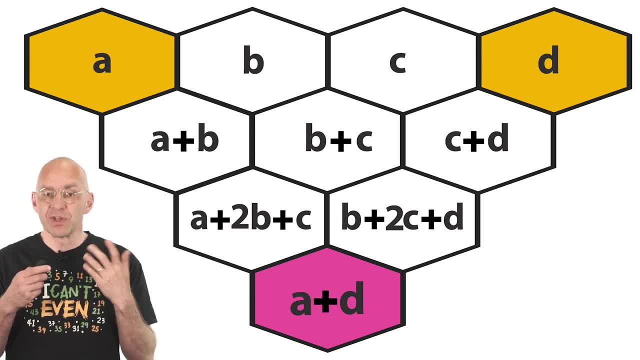 here turn into pluses And again the three times, some things in the bottom hexagon disappear. So for this Pascal three color game as well, the number four and therefore all those other numbers, 10,, 28,, etc. are special. What about the odd, even black, white mod two Pascal game? In the case of this game, 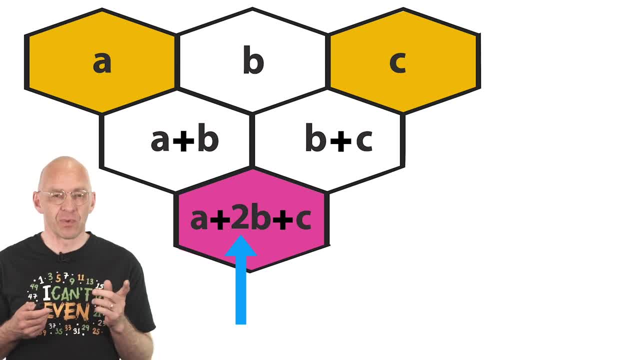 we only need to worry about the smaller part of the triangle. Why? Because two times anything is even, and so it reduces to zero mod two, And so the two b term in pink zaps to zero. This proves which three is special for the. 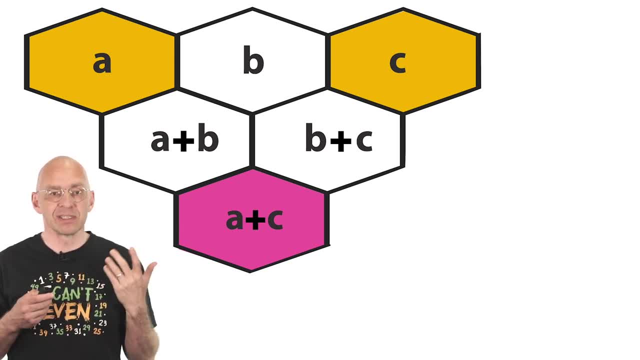 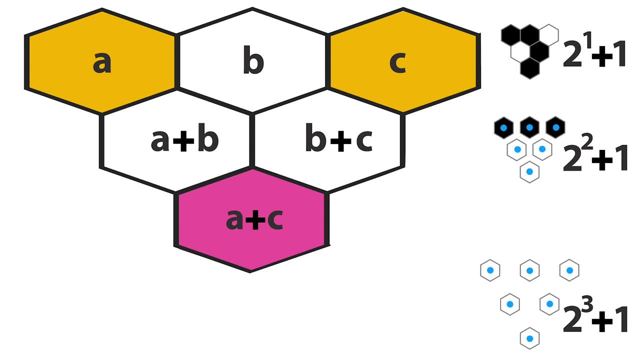 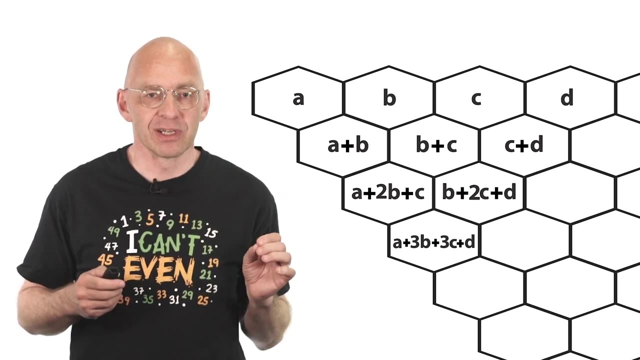 mod two game, And then by our collection argument we can see that all powers of two plus one are special. Of course we can play the same games using any number of colors. With m colors we can then use the sum modulo m or the sum modulo z, And then we can use the sum modulo m or 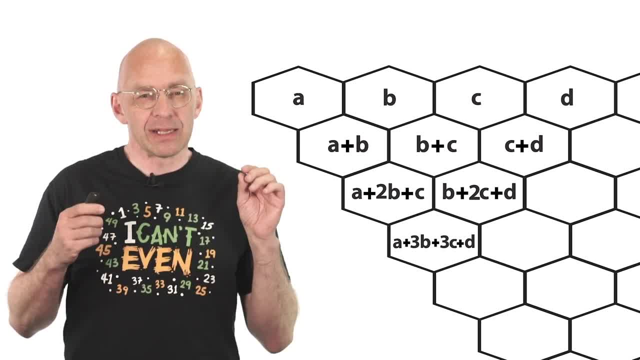 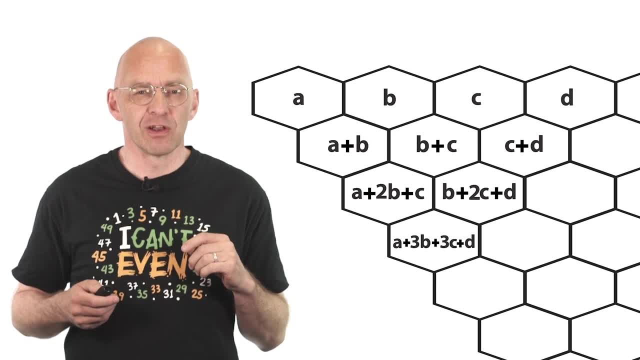 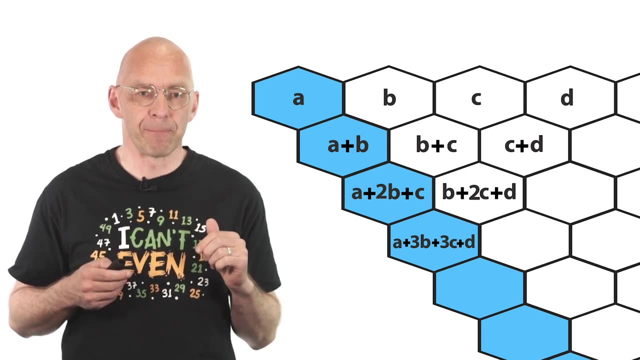 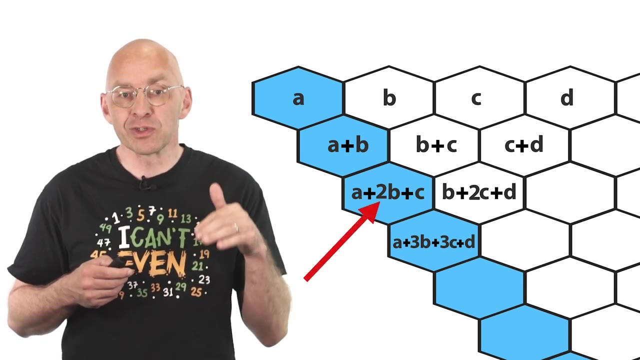 its negative as our generation rule, And then the same algebra and our contraction argument can pin down the corresponding special numbers. For this we need to identify those entries here for which all the middle coefficients are multiples of m, As we've already seen, for m is equal to two. the first time this happens is here, And as we've also already, 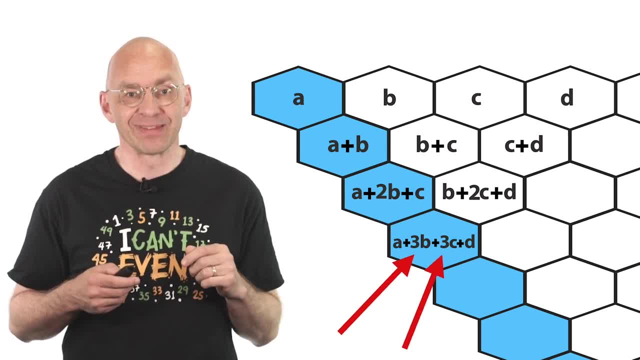 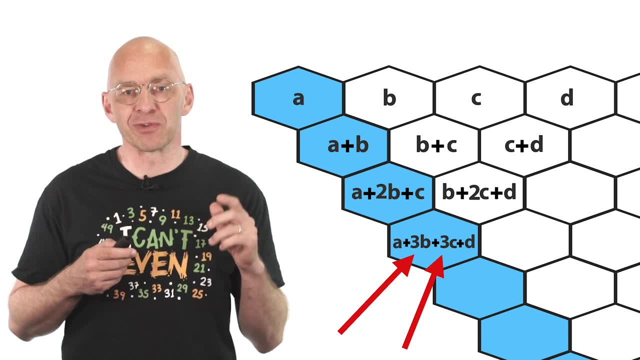 seen, for m is equal to three. the first time this happens is here And now. a challenge for you, A tiny little challenge: Figure out the smallest non-triple special numbers, for m is equal to four, five, six, etc. until you get sick of it. A hint: 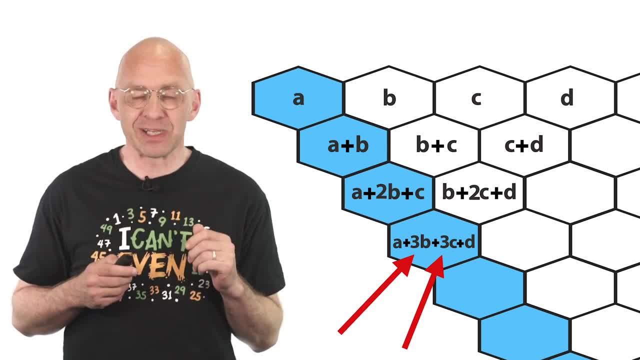 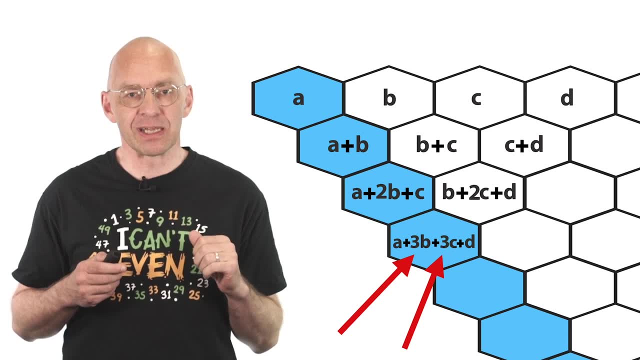 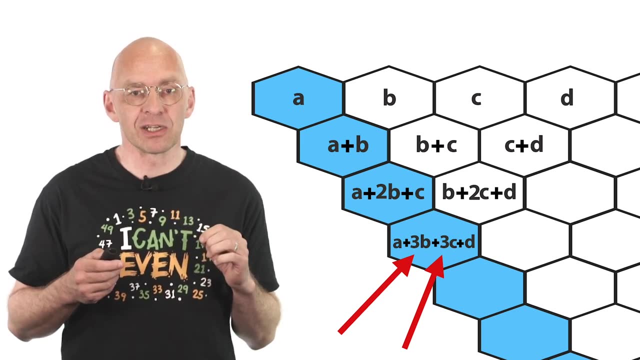 Just focusing on the blue entries, Can you see another Pascal triangle? If you are keen to learn absolutely everything else there is to know about these games, check out the intelligence article by Erhard Behrends and Steve Humble that I mentioned earlier. In particular, in this article you can find a 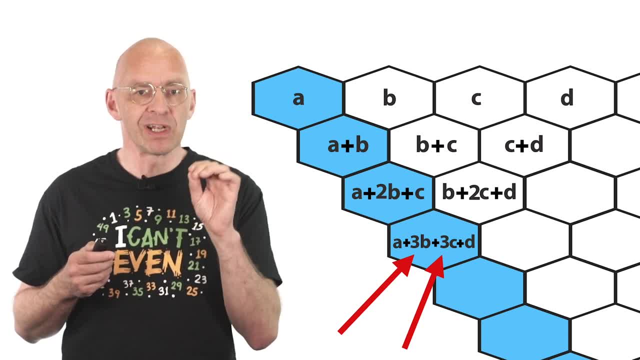 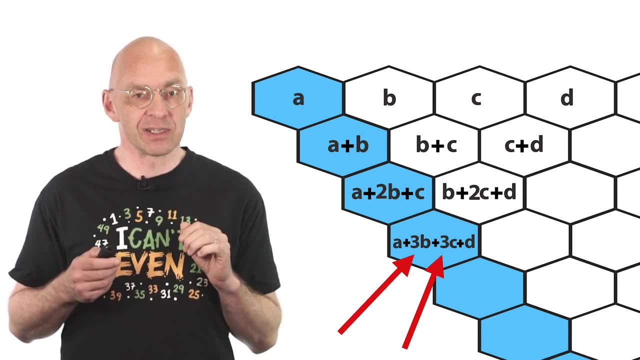 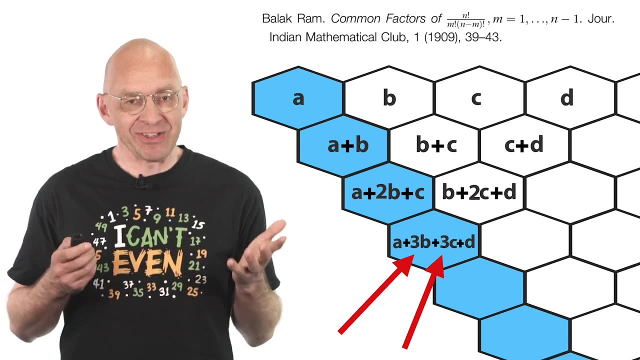 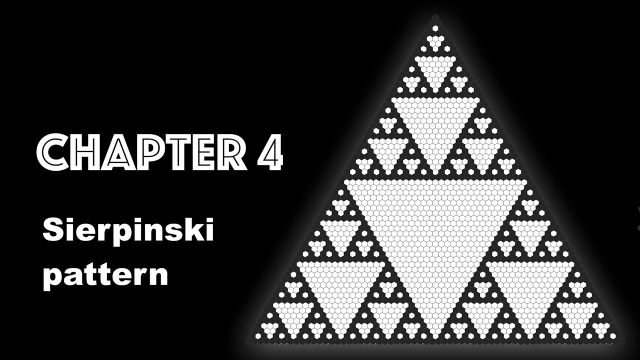 proof that the special numbers we've spotted are really the only special numbers. This proof is based on a 1909 article by the Indian mathematician Balak Ram in the journal of the Indian Mathematical Club. How on earth did they find that one? 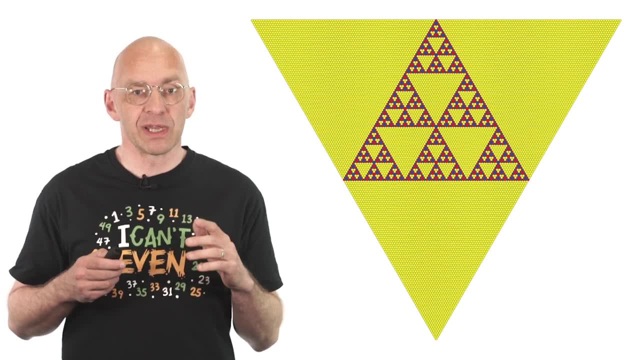 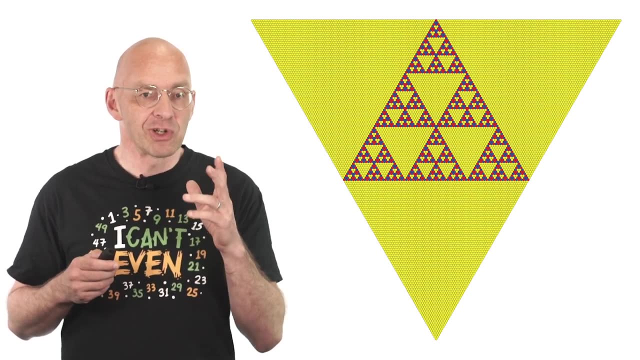 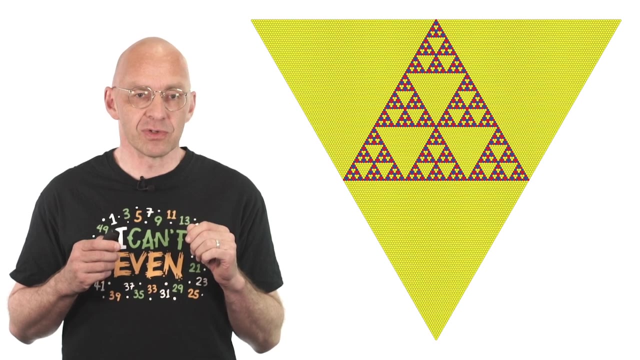 Using the special numbers that result from our addition rules, we can fashion ourselves some nifty keys with which to explain those striking self-similar patterns. Let's have a closer look at the triangle over there. A reminder: We got this triangle using our original three color addition rules, starting from a row of yellows with a single. 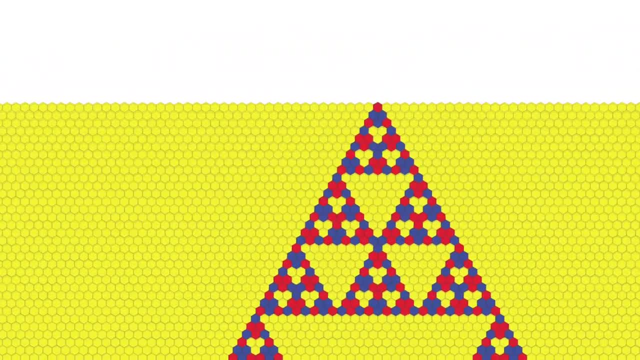 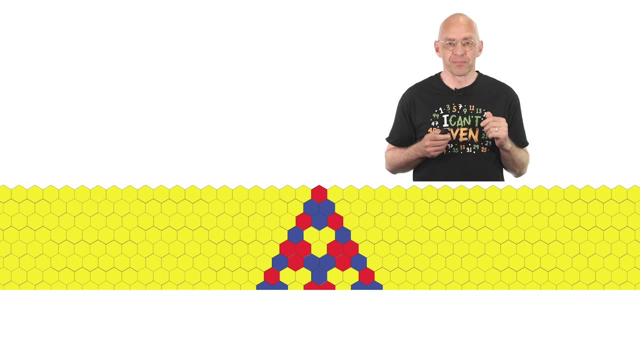 red hexagon right in the middle. Ok, so the whole thing starts with this row of hexagons at the top. If we do that, we now have two with yellows that we can use to round around. We ask ourselves: why is these hexagons so huge? 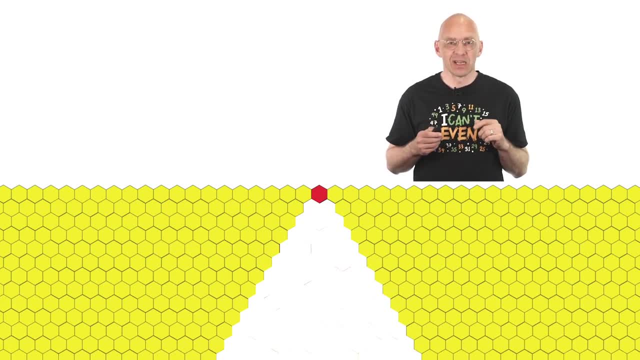 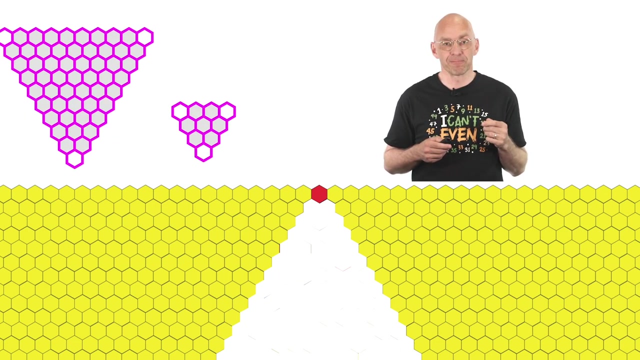 This sentence means that there are two yellow ships, both in the middle pharmaceutical economy page dot do. In order to do that, I make myself one template each for the special numbers 4,, 10,, 28 and so on. I now place the template. 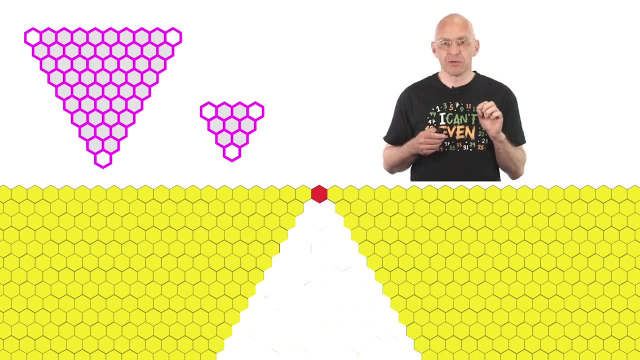 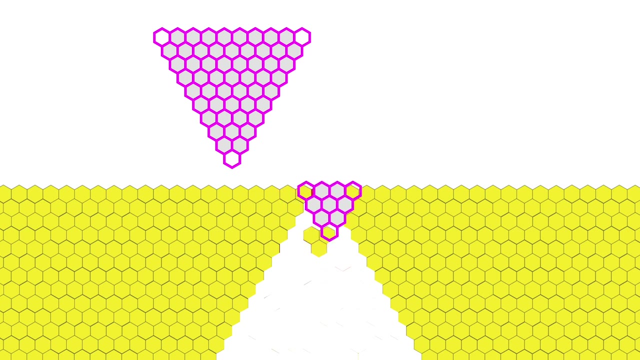 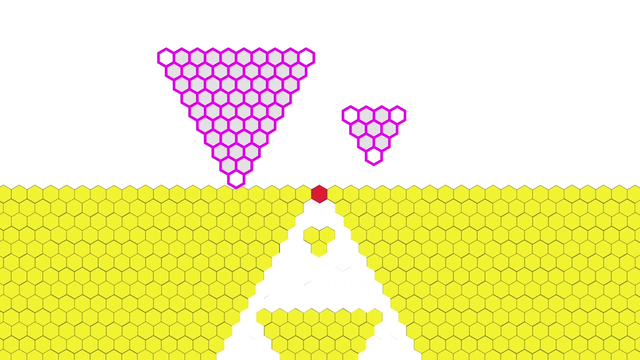 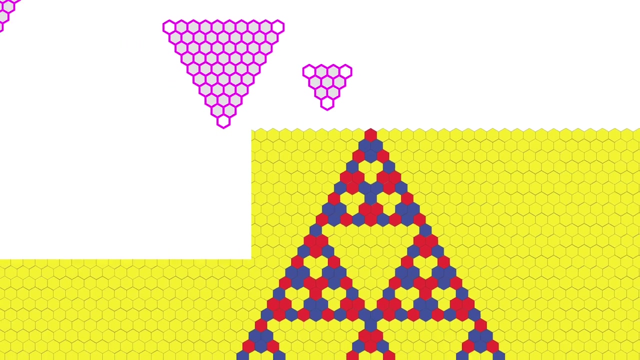 so that the two upper corners sit on yellows in the outer regions. Whenever this is done, we know that the bottom corner of the template might also be yellow. Let me show you. All makes sense, right, But just to pinpoint exactly where the self-similarity of the pattern. 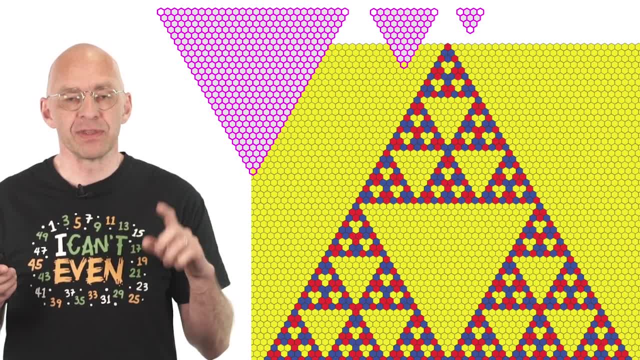 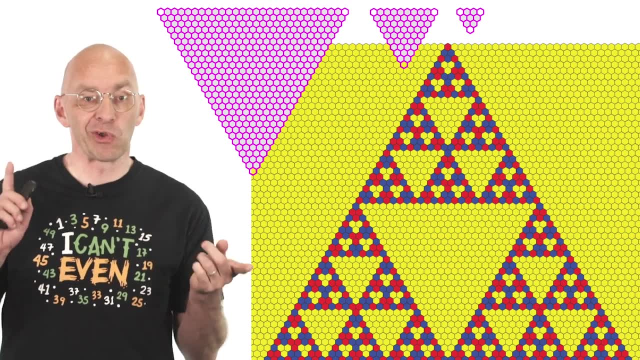 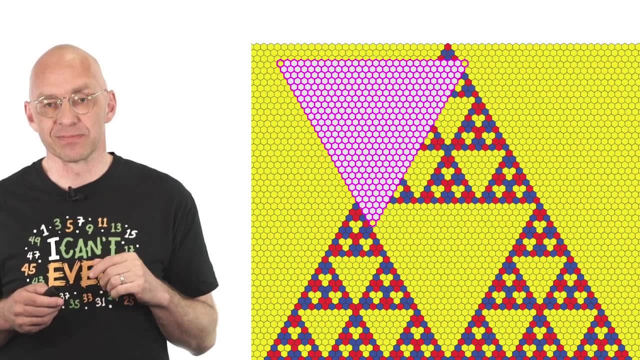 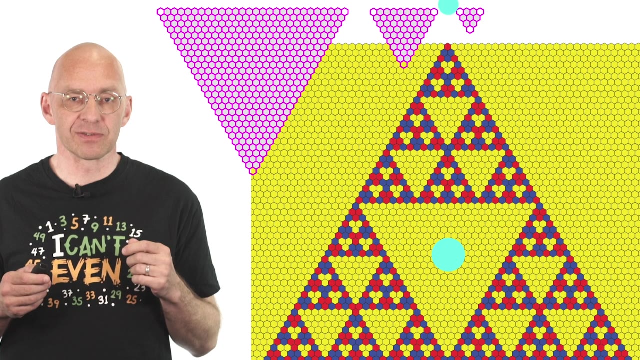 comes from. think about the yellows being built in this order. When we place one of the templates so that its top two corners lie in the left and right oceans of the yellow, the template should look like this: This takes care of all these centered triangles, But now focus on this off-center region here. 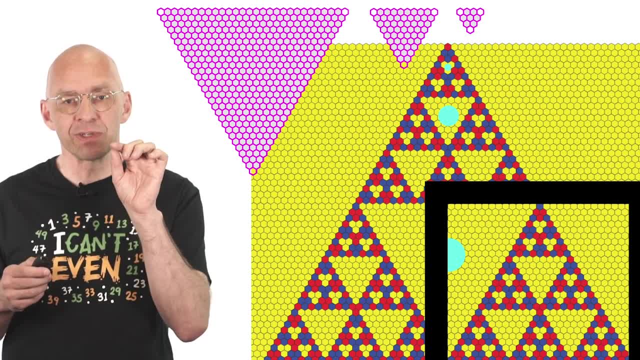 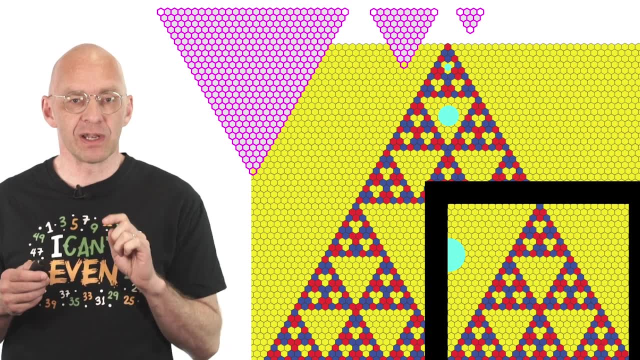 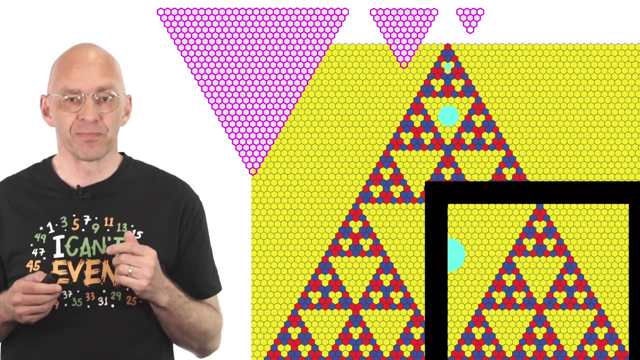 What's happening here? Well, we already have large lakes of yellow on the left and right, plus a starting row- all yellows with one hexagon of a different color in the middle. So within this frame, we can now generate centered triangles, exactly as before There, And so on. 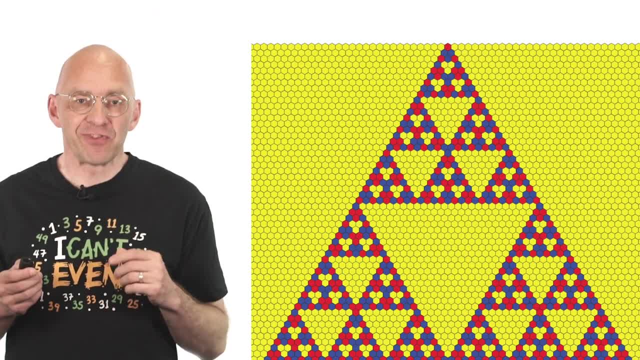 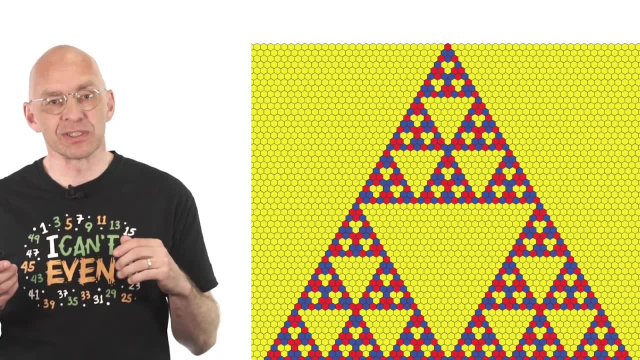 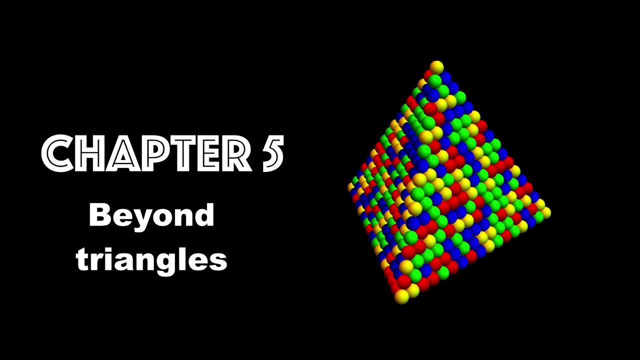 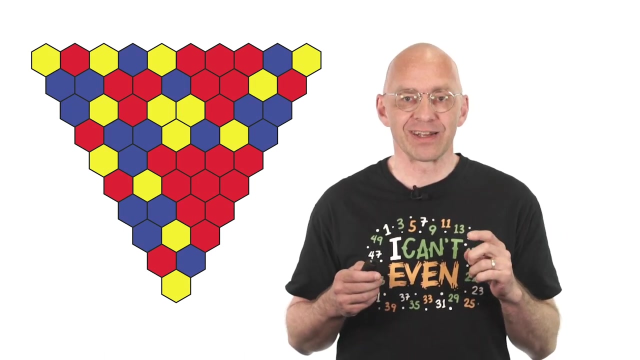 This really gives a very good intuitive feel for where this self-similar pattern comes from, doesn't it? And it's not that hard to turn this intuition into rigorous proofs for the fractal nature of these patterns. So let me show you. There's one very surprising feature of the original three-color game that I did not mention yet. 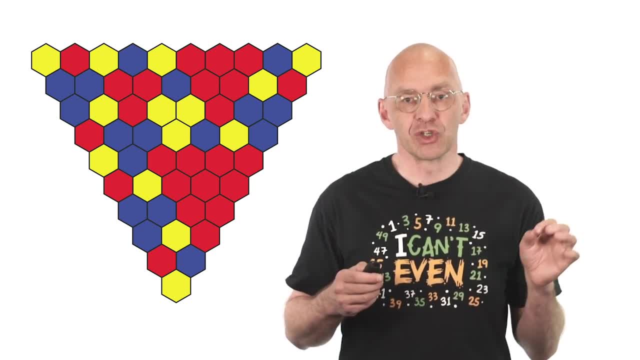 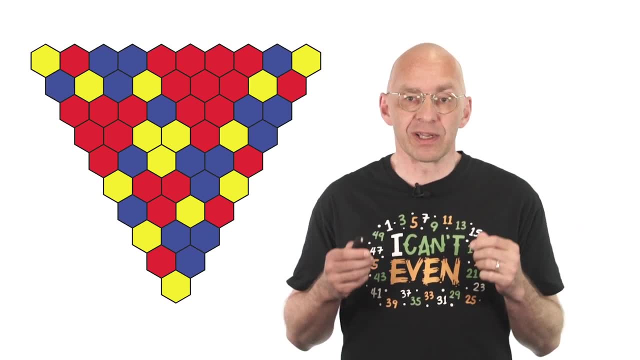 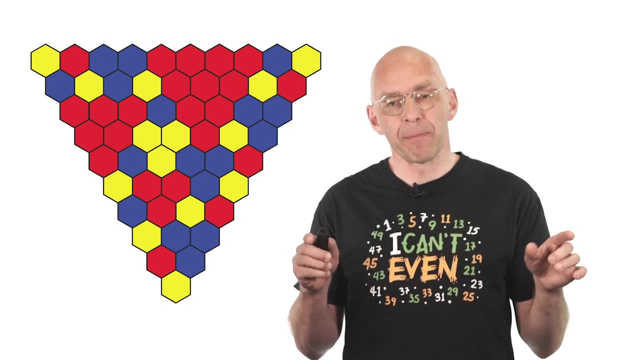 When you rotate one of the triangles colored like this, you get another triangle of the same type, So what this means is that this new triangle also grows from its first row. This feature is shared by all the other negative mod M colorings, but not the other three-color games. 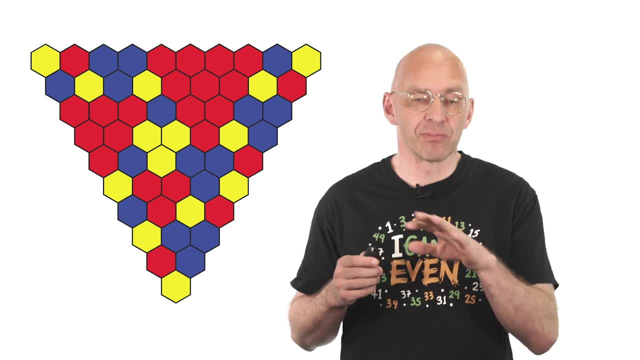 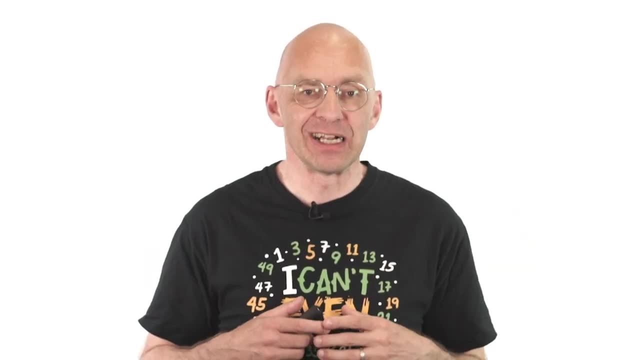 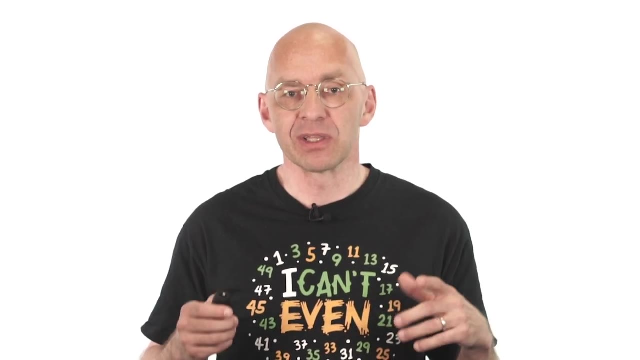 But it's straight. Pascal, mod M, colorings Except mod 2.. Can you think of a simple explanation for this phenomenon? Anyway, to finish off, let me just show you an animated introduction to the most natural three-dimensional counterpart of Steve's three-color game that also shares the 3D.